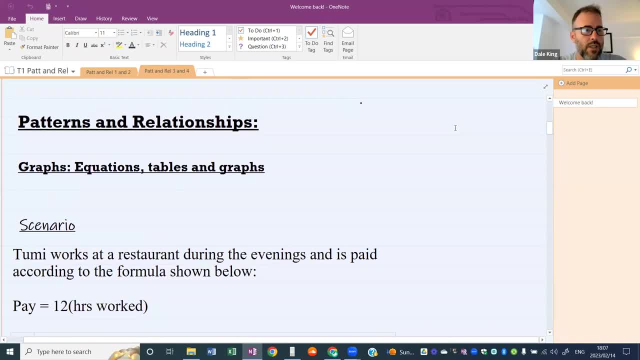 going to start off with an easy one. here's a scenario so to me. works at a restaurant during the evenings and is paid according to the formula or equation shown below. now you can see here that we're using words, not variables, because this is math lit. we don't want to think like we're in commerce, we don't like those things, so we've got pay because. 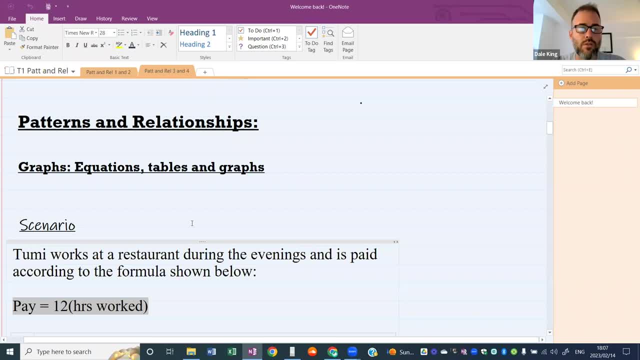 to me is: pay to get that. you need to take 12 and multiply it by the hours that are worked. okay, so that's the formula. so pay to get paid: this equals 12 times the hours worked. just remember, when you have 12 in front of a bracket like that, then that means you need to multiply by what's. 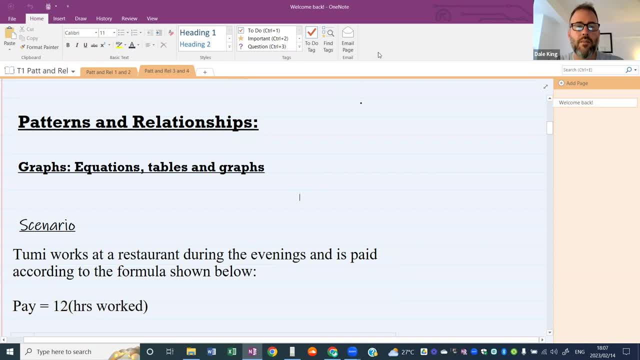 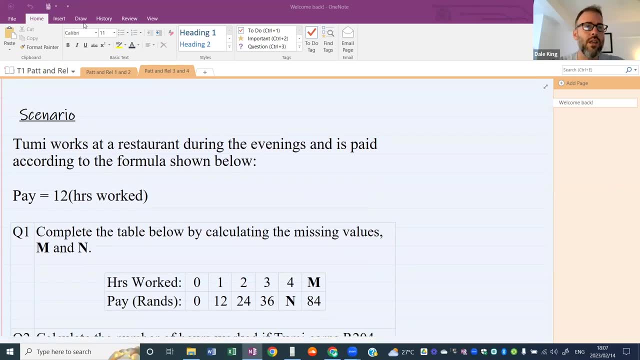 inside the brackets. okay, um, all right, so let's get started. here is the first question, and you guys are going to get stuck in from the word go making you work from the beginning. so hang your pen and paper reading your calculator. it says: complete the table by filling in the missing values m and n. look carefully at the 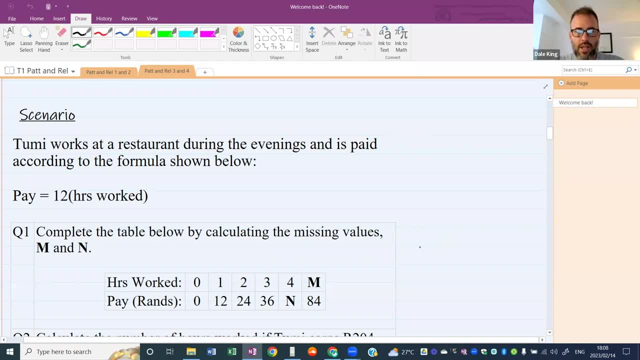 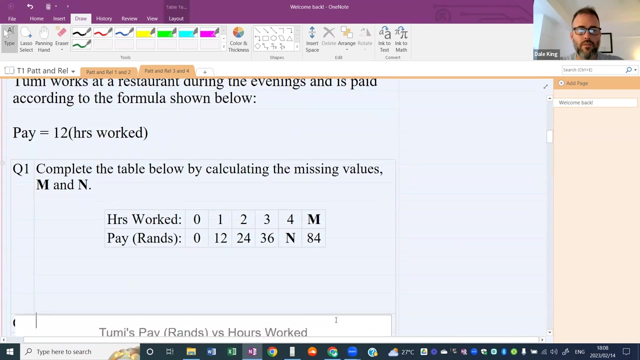 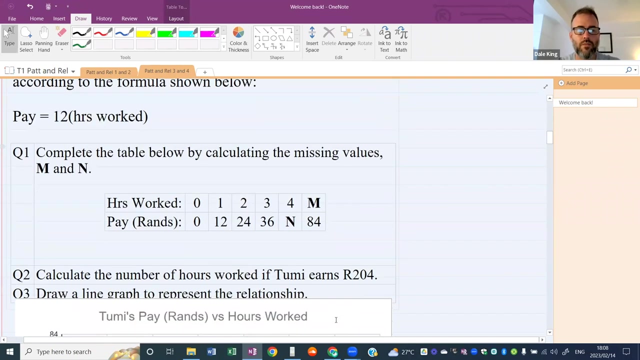 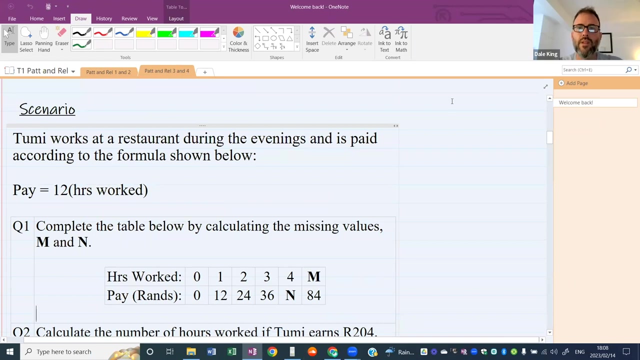 table. don't be tricked. we need to work out m and n. all right, I'm going to give you two minutes to do this one and then we're going to try it ourselves. off you go. oh oh, phyllis jordan, too fast. all right, we got people with answers coming in. um try, make sure that you guys get your. 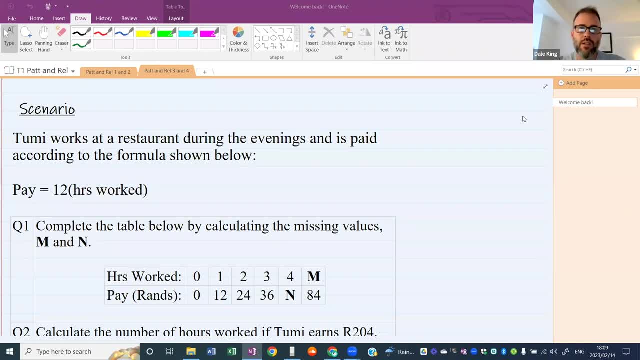 own solutions, don't look at the ones that are popping up. try and make sure that you get yours right on your own. let's see how you do with the calculations. so all right, the answers are coming in thick and fast. let's have a look. let's have a look. let's see how we do this. 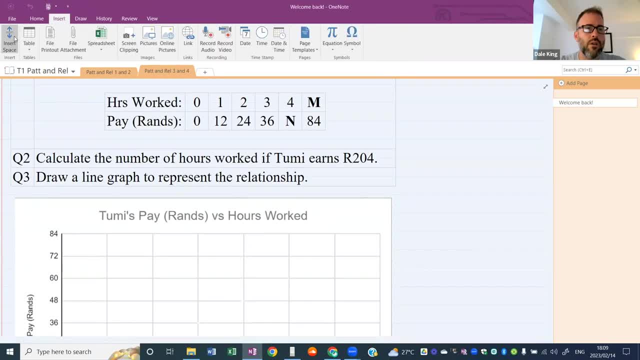 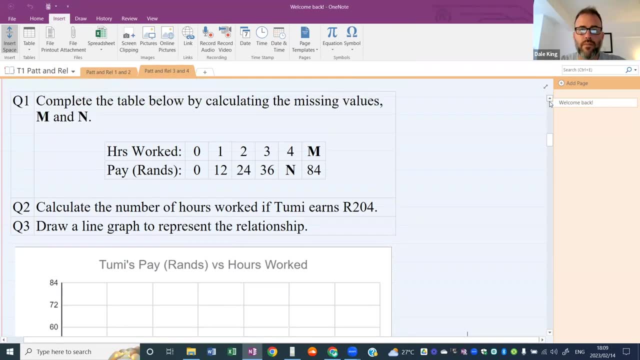 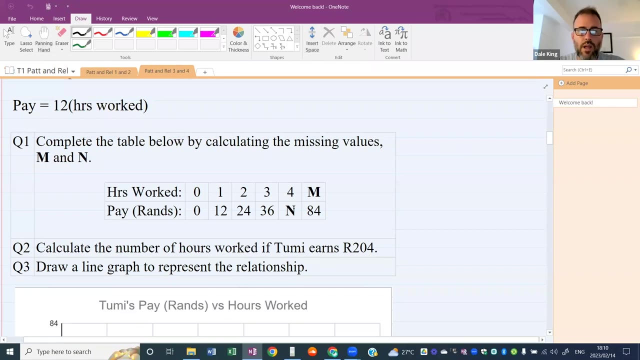 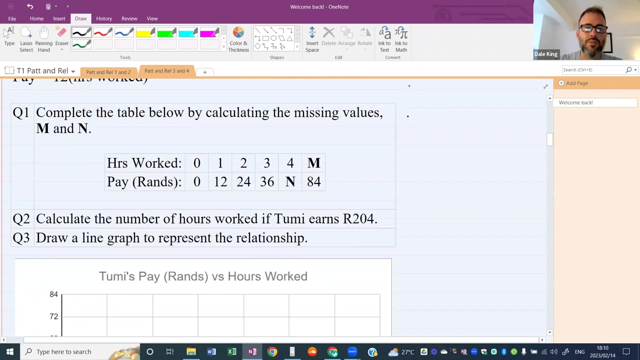 all right, i'm going to create a little bit of space down here for me to work. let's do it on the side, okay? so the first one i want to do is i want to work out in this one over here. all right, so to work out in which is pay, i can actually use the formula, because formula says pay. 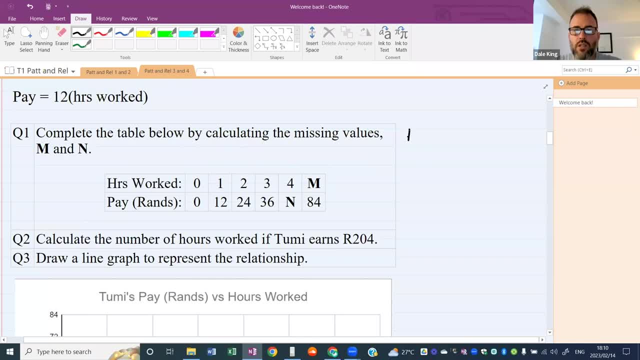 is equal to 12 times the hours worked. so i'll use the letter p here for pay. i'm going to write the whole word out and i take 12 and i'm multiplied by the hours worked. now the hours worked. if i go straight up, there's four, so i can substitute four in there for the hours work, and we should. 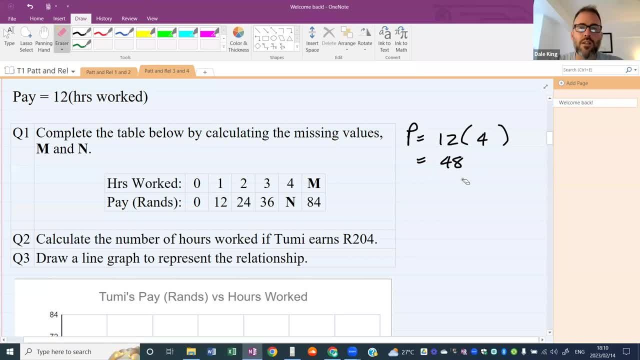 get an answer of 48, and i know kia is going to say something now when she sees: go forget to you units. all right, so the units are ran, so we need 48 rads. okay, so that's for m. okay, so we should say, in fact, if you wanted to replace p for m here, it's fine, but m equals 48 rad. all right now, sorry. 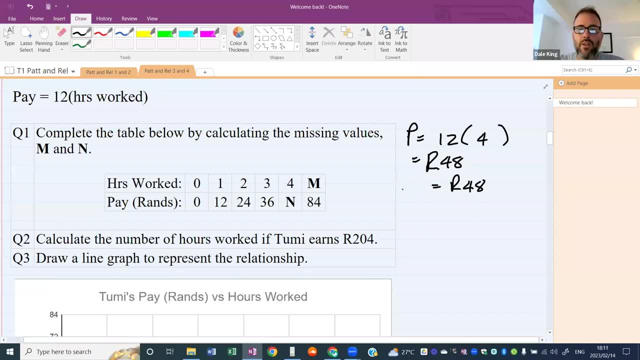 that was m, not m. okay, now we're going to move on to m all. right now, m is hours worked. okay, this is hours worked. so if i take my formula again, p is equal to 12 and then open the brackets here. now, instead of substituting in the hours worked to get my pay, i'm looking for this hours. 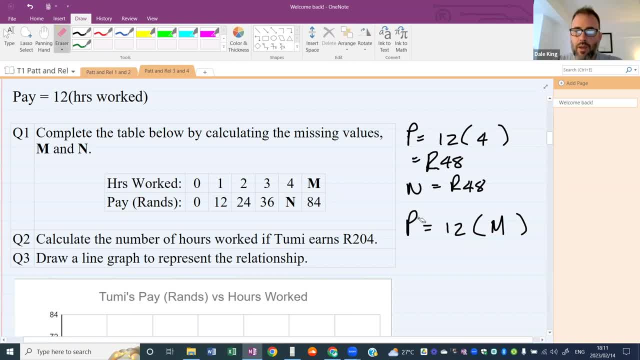 worked. i'm going to call it m for now. all right, and on the the p side of the formula, they give us the pay value, so they tell us that the pay value is 84 rad. okay, so to get m here, i just need to get rid of that 12. how do i get rid of that 12? well, it's attached to the m with multiplication. 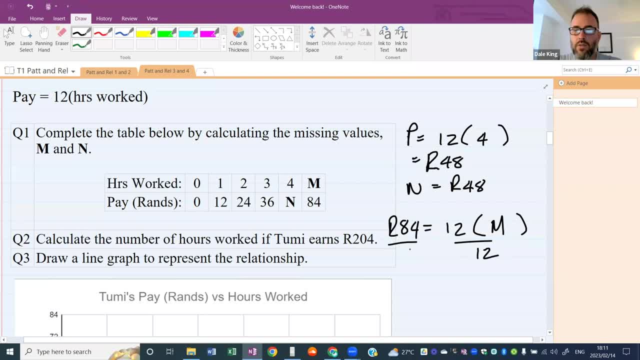 so i'll do the inverse operation. i'll divide both sides by 12. okay, so m is equal to 84 divided by 12, and that should give me seven, if i'm not mistaken. all right, so m is equal to seven. so she has to work. uh, to me, has to work seven hours to get 84 rads. okay, okay, it looks like the answer. 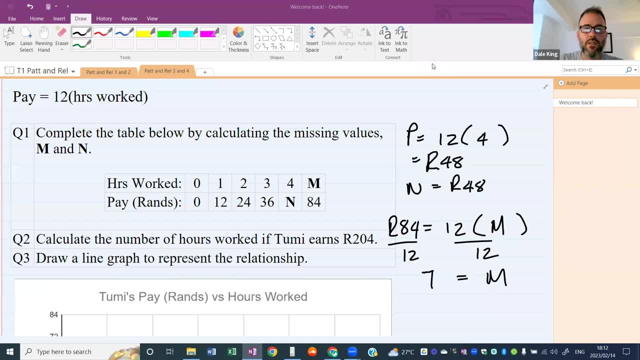 is yes, so i'm going to do the inverse operation. i'll divide both sides by 12. okay, so m is equal are pretty good. yes, we are off to a fabulous start. we're off to a good start. okay, phyllis is a god. sorry for this. 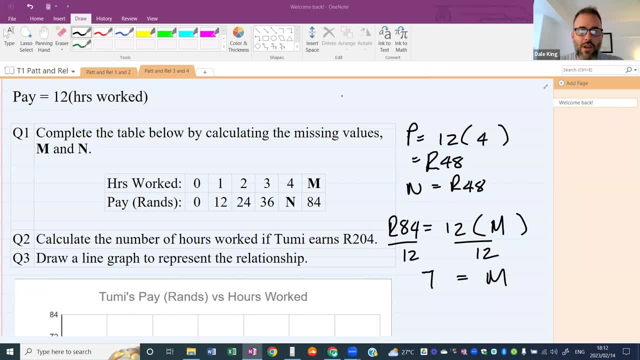 all right, but this is not a girl, it's a guy. all right, here we go. so we're going to move on to the next step. now we need to work out- i'm going to remove this. if you need to uh at any point, uh as you're doing this lesson. if you need to uh, save the calculations. you want to have a look at them. 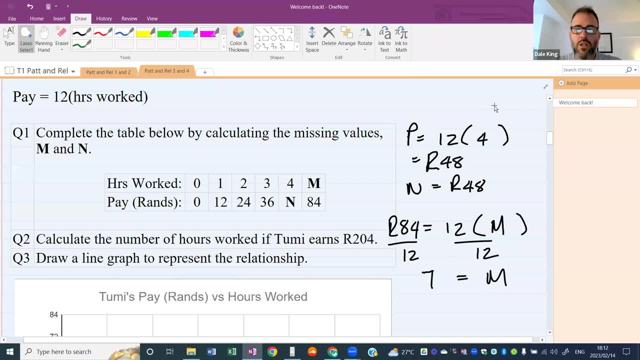 later. if you're using a laptop, you can use the print screen function. uh, it'll copy the image of the screen and then you must paste it somewhere else. or if you're on your phones, uh, just take a screenshot of the calculations, because i'm going to remove them now, just for some space, okay. 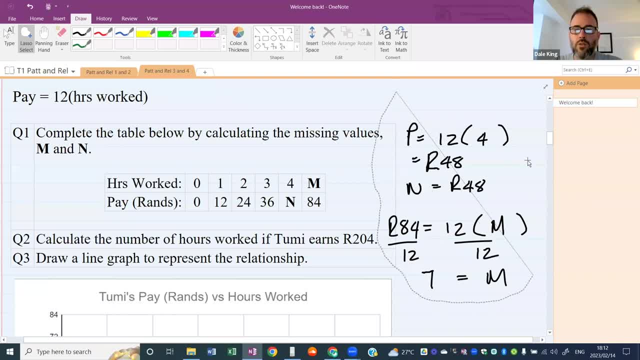 all right. so let's remove this because we're going to answer the next question. next question says: calculate the number of hours worked. if to me earns 204 rad, all right, let's see how fast you guys can do that. how many hours the to me work if the pay is 204? 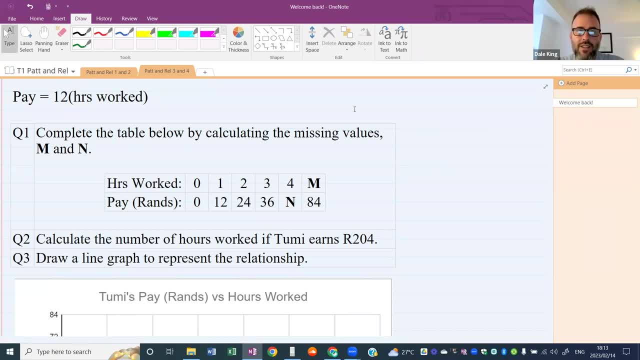 come on so fast. you were still explaining and then an answer popped up. i was like, wow, these guys and girls, oh my gosh, as soon as the next question comes up, they want to do it. it's fantastic, it's enthusiastic, brilliant, yeah, no, i think every day should be. 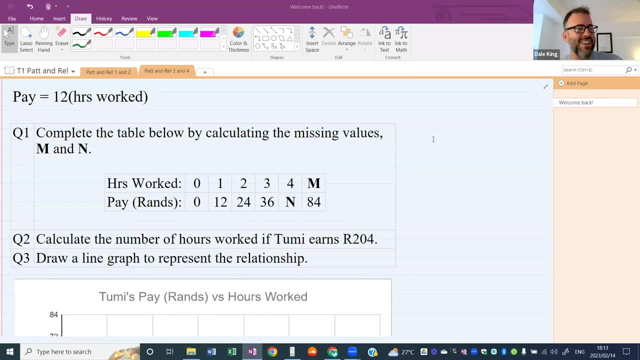 valentine's day. everyone's got energy and they're excited, they're buzzing. i hope everyone had a good valentine's day. all right, we've got some answers coming up. okay, let's have a look. let's see if your answer is the same, all right, so calculate the number of hours. if the pay is to me earns 204, so that's pay. 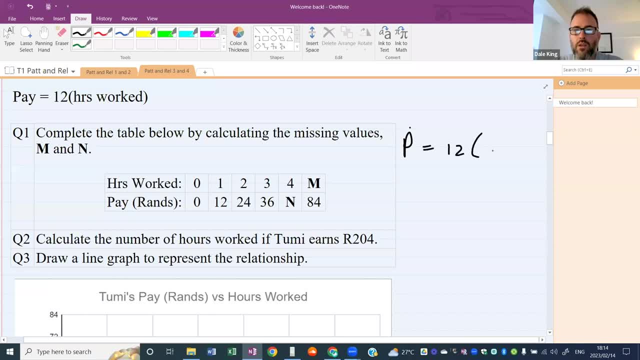 so to me is paid 204. okay, so in my formula i'll put you at h4 hours or hrs for hours, how many hours if the pay is 204? so 204 has to go on this side of the formula and we need to work out the hours. 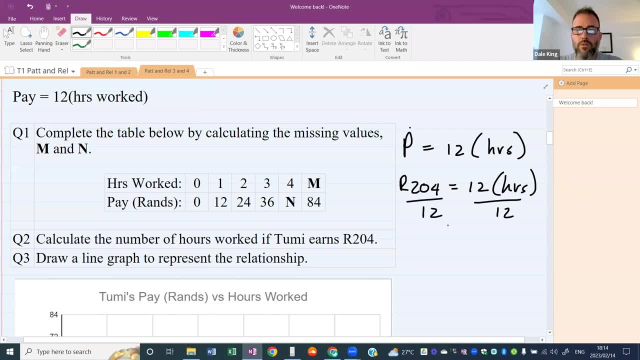 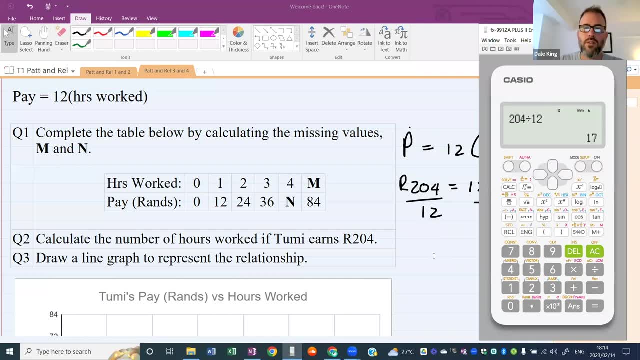 again, we're going to divide by 12, divide by 12. i'm feeling lazy, i'm going to get the calculator to do the work for me. so 204 divided by 12 gives me 17. very good, all right. so the hours that, to me, worked. 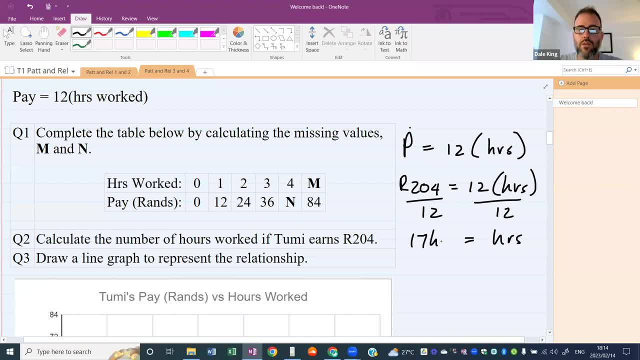 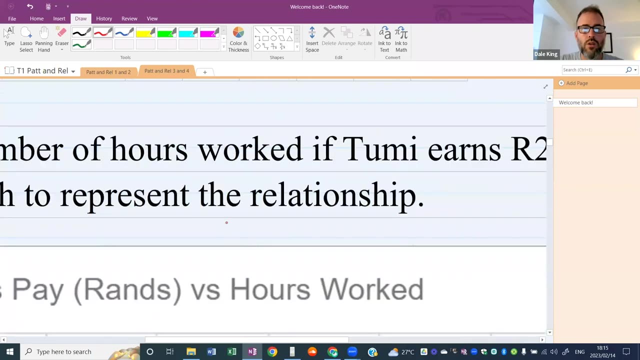 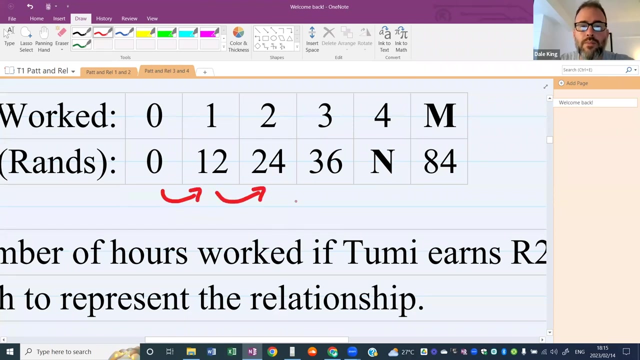 17 hours. okay, all right, so we're learning how to use the formula here to help us get the answers, which is fantastic, and in the previous lessons and what we did was we also when we asked to solve for these unknown letters here. what a lot of you guys at the beginning was. you noticed there was a pattern. 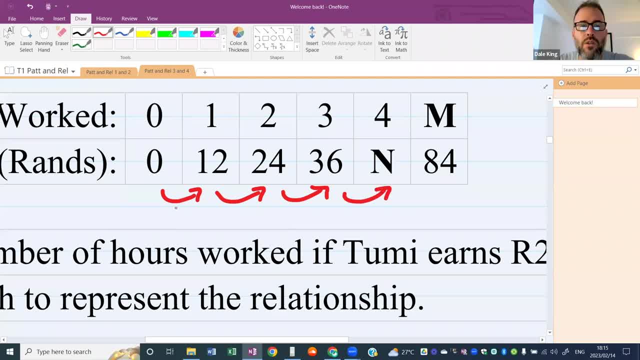 every single time, which is adding on 12.. okay, so some of you might have used that method where you add on 12 to 36 to get the value of n, which is fine, as long as you can see that all these numbers go up by one. 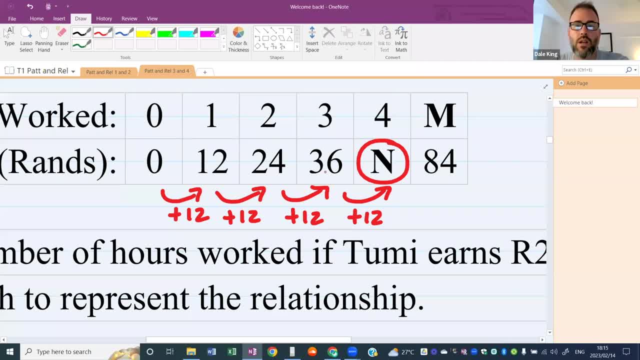 then you can find n's value. if i think these numbers go up by one, then you can find n's value. all right, because it's a constant difference. okay, uh, but it poses a problem with 84, because 84 doesn't form part of the pattern, so you might jump a couple of times to get to 84. but if that, 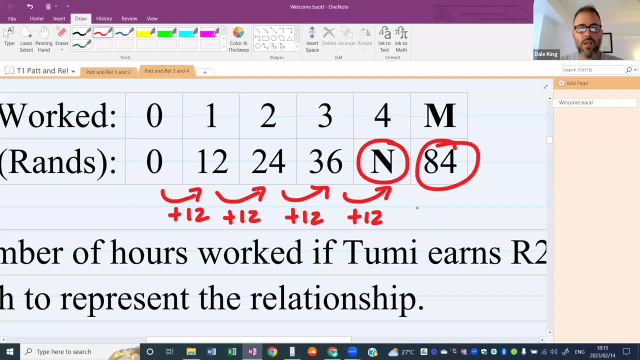 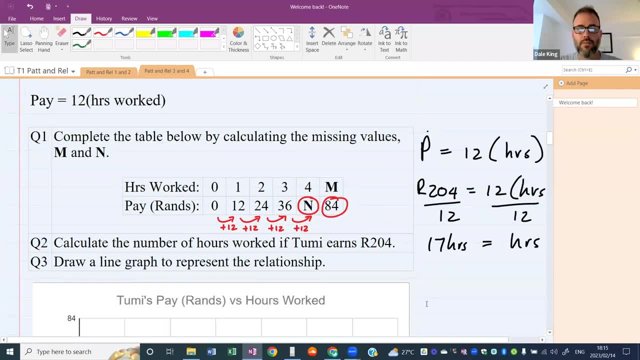 number is really really big. you're going to do a lot of jumps to get there, so a formula really really helps in these situations. okay, so try and learn how to use the formula substitute in, change the formula around to get things that you need. okay, now you guys aren't going to really be. 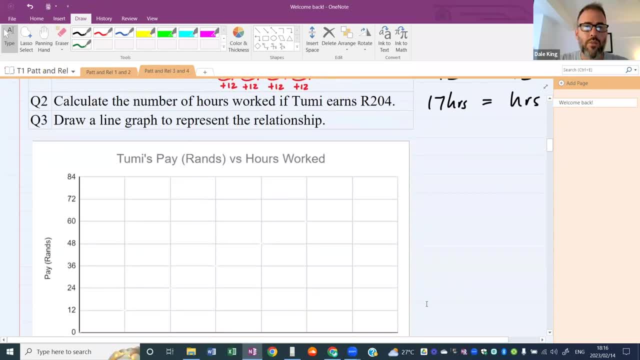 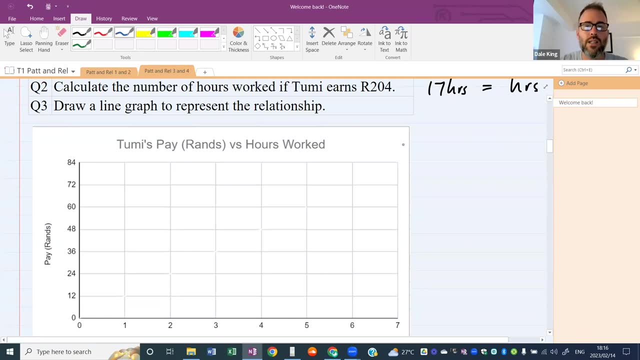 able to do this one, so i'm going to do it for you. it says: now draw a line graph to represent the relationship. okay, so we're going to use the table of information to help us plot a graph here. i'm going to use blue for the line um. before i draw this line, can someone please put in chat? 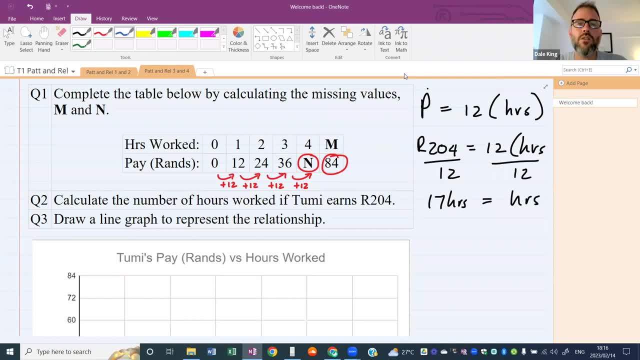 what type of linear graph are we going to see? we learned about these last week. i know peter is very good with this. uh, we are, we got 17. hey, if you turn it forward about about 12 is 17. check your calculation. um, all right. what kind of linear relationship? is there a linear? 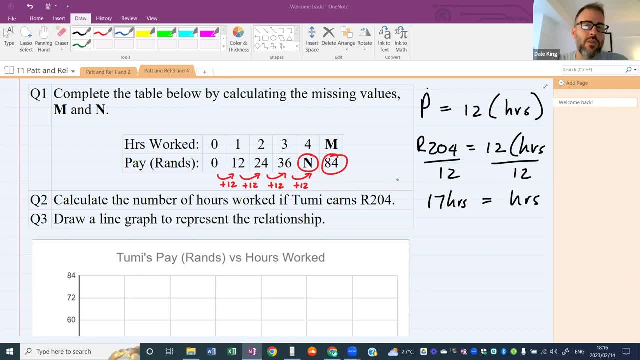 relationship. but which one is it? i don't know if you guys can remember the names from last week. where is it? he usually is quick with these answers: yes, they're quiet. now, there we go. computer says they can't see the graph. you don't even need to see the graph, we don't even need to. so if you look at the table, 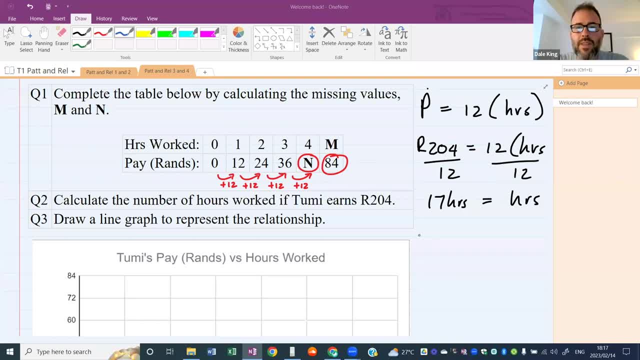 that should give you a clue as to what kind of graph it's going to be. it is linear, so i'm telling you it is going to be a line graph, but which one? there were a couple that we learned last week. oh, they've forgotten everything. you see, this is what valentine's day does. 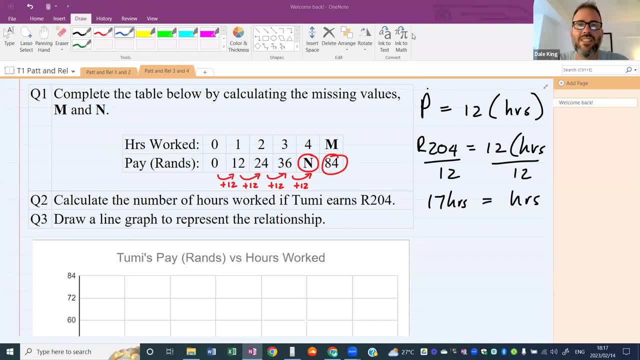 this is with your brain. i was only you missing a few words there. all right, so direct, yes, it is a direct relationship. uh, proportional relationship, it is proportional. yes, fixed, fixed is the one that goes horizontal for your. yes, direct, proportional, good, okay, and there was another way. it said there were two words. i was looking for constant something. 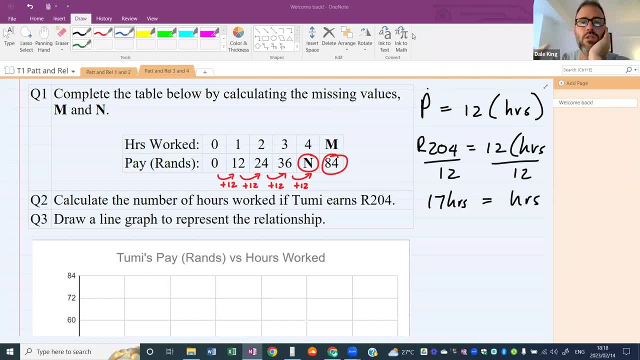 right, the direct proportion is correct. you also could use the words constant something. yes, direct proportion is good. constant something, not constant fixed. ah, who was first there? oh people, well done, constant increase, good stuff. we are well done. constant increase, okay, and these administrators are also with the answer. all right, so it is a. 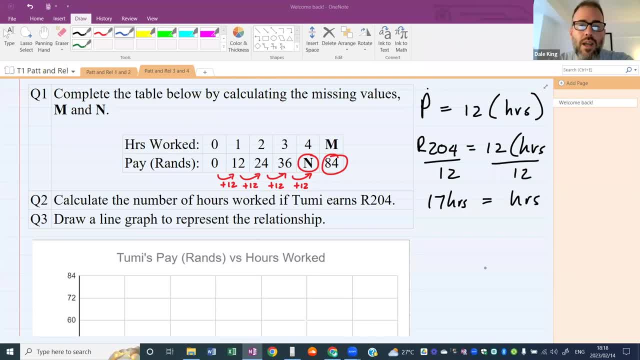 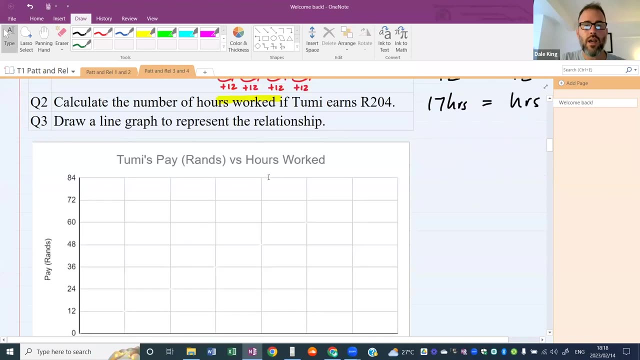 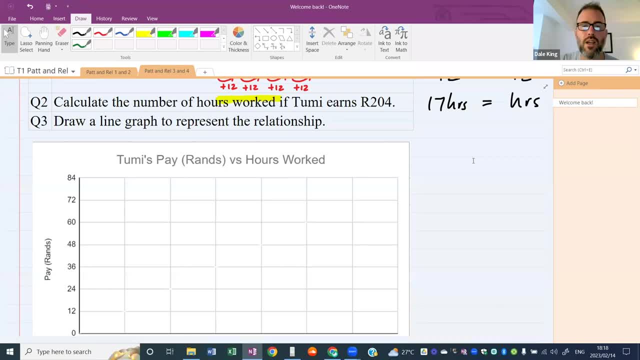 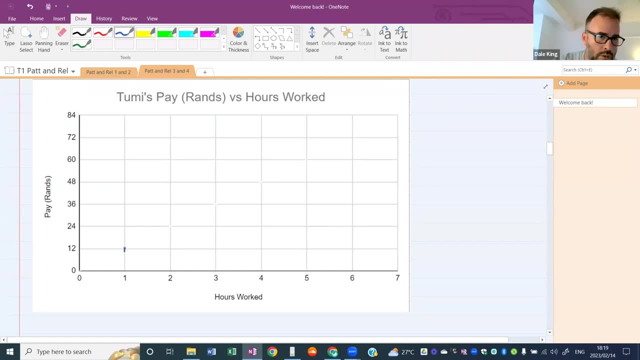 between the values and it's good, so it's a constant increase. okay, so how does it look on the the axes? well, for one hours worked, we got 12.. so i'll put a dot there. for two hours work, we've got 24. for three, we've got 36. for four, we've got 48 and the table we had to calculate five. 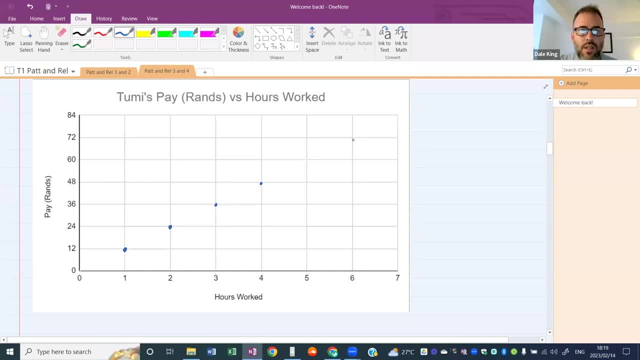 no, we didn't have to calculate five. we were going to skip those two because the table didn't have them. i'm going to go to seven for 84, because we worked that out okay. so i've got all these dots here. now i'm sure you can see how these dots are all lining up all right, and 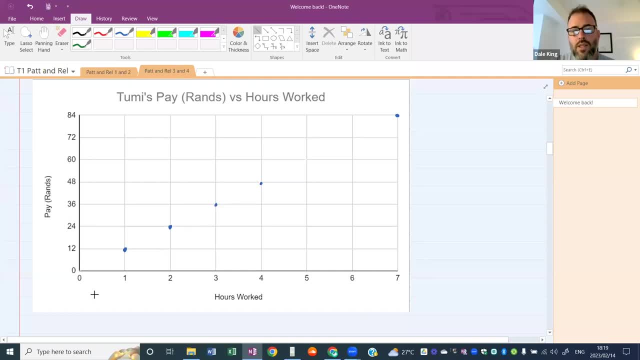 do we start from zero? well, let's think about it. if it truly doesn't work any hours, then she won't get any money, so she won't get any pay. all right, so we can start at zero. so i'm going to start at zero there and go through all these dots and line them up and draw a line. okay, now just a hint. when 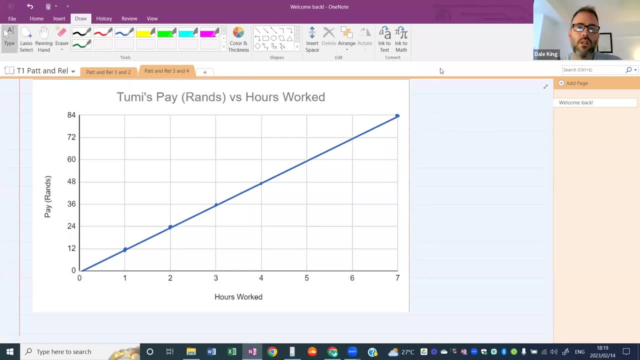 you get one of these tables and you know it's the constant increase for direct proportional relationship, you need to check your line, okay? so sometimes what the guys do is they might make a mistake in the table and then they draw that mistake onto the line. so what sometimes happens is maybe: uh, let's do the last. 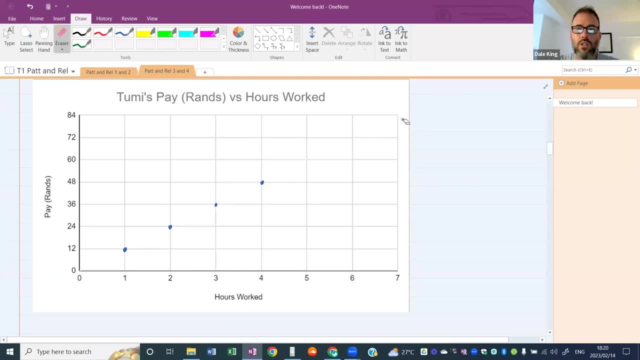 one. so maybe the last calculation that you did, or one of the questions, didn't give you 84, but gave you something like 64 or 65. okay, then you'll see that this graph doesn't go up exactly straight. if you join the dots you might stop there and then you might draw another line to that point that you calculated. 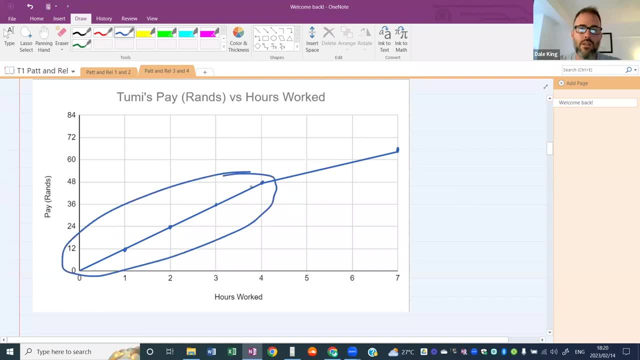 okay, so these values are all given in the table and then this one over here is the one that you calculated. so if you, if you know this is why it's important to recognize it's a constant increase for direct proportion, if you know it is that kind of relationship, then it should go up straight all. 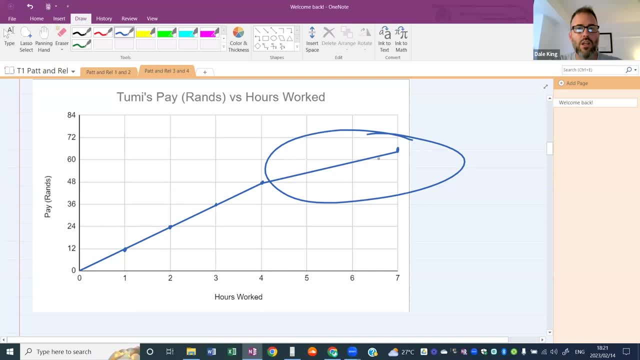 the way. all right. so when you see your graph do this, you need to go back and check your calculations for one of those questions, because it should go up in a straight line, okay, so that's a way to help you check if you've done your calculations right. so in this case, we know it's a a direct. 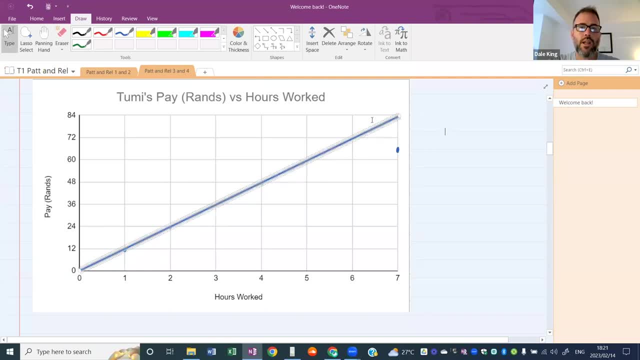 portion relationship. so it should go straight up in a line like that- a straight line- you shouldn't have to move your ruler on one end all the way to the top- should be a straight line, okay, um, all right, so let's move on. we're going to change it slightly now, okay, so have a look at this graph: direct abortion- constant. 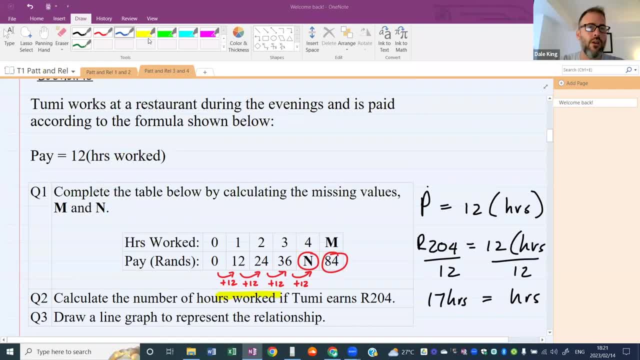 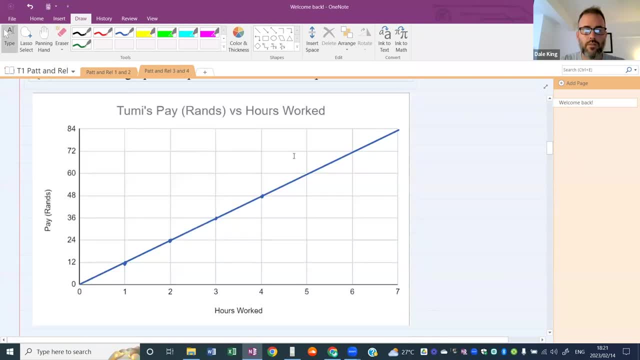 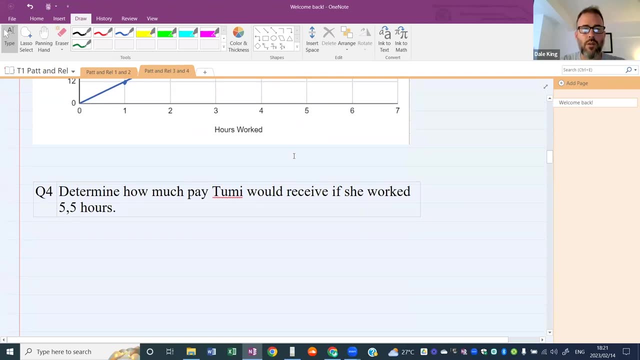 increase based on this formula that we had over here. so that's what this formula gives us on the graph. now we're going to move on to a new scenario. well before that, let's do this, let's do this: determine how much pay to me would receive if she worked five and a half hours. let's just quickly. check that, because now, this is the you know, this is the you know will be crossing one of these lines here is looking at you. know how much loss is looking at you if she worked five and a half hours? let's just quickly check that, because now this is this is 179 years of flow quantity video data used. i mean, are you crazy? i think it is exactly right. we're going to change it slightly now, okay. 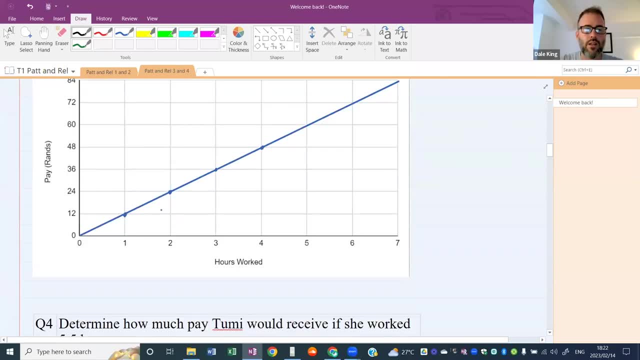 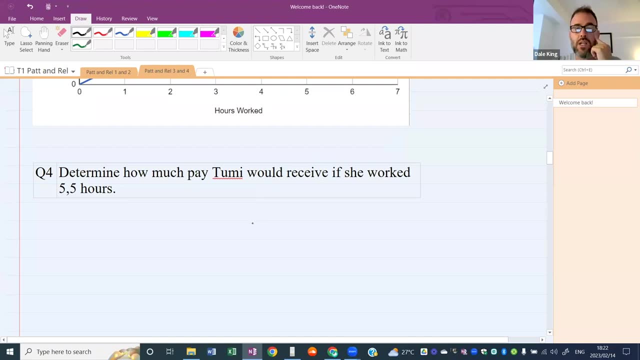 different to the other ones. we've got a decimal hour, all right, so determine how much to me would receive if she worked five and a half hours. can you quickly do that calculation and we're just going to check decimals and how they affect our answer- how much pay for five and a half hours? 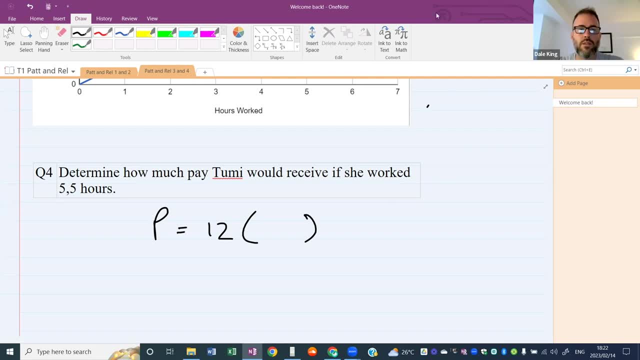 i'm sure the calculators are working now. okay, we've got user with 66, 67, 66. all right, looks like we've got an answer. okay, let's quickly check. let's see if 66 is correct. all right, hold on to your answers, let's have a look. so we're going to substitute our hours, which are: 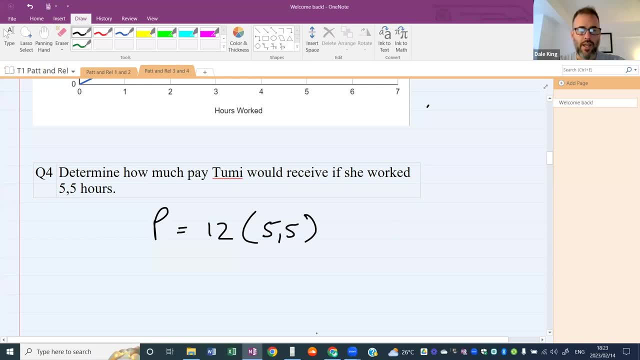 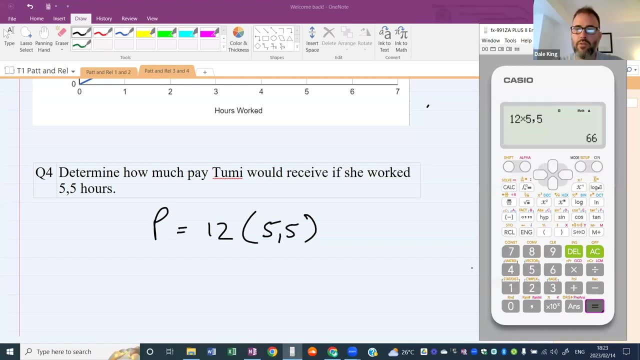 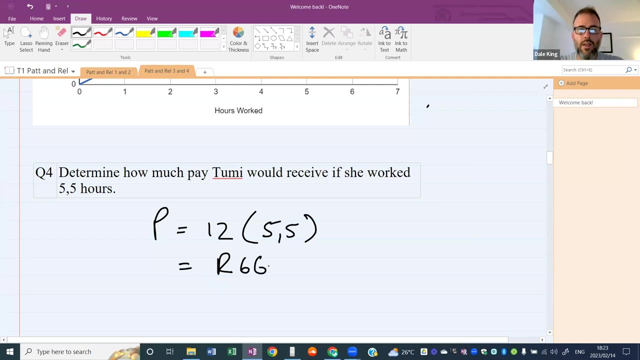 five comma five, excuse me- into the formula. and then, like i'm sure you guys did, we're going to use the calculator just to make sure that we save times 5.5. and yes, the calculator doesn't work for us and we get 66 rands because this is pay. okay, we get 66, right, all right, 66, yes. 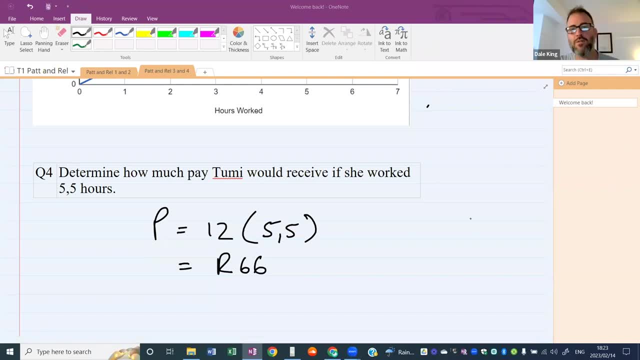 who is that? was it? ah, jill, aren't they? 66? that is what i'm laughing at, like: wow, please, guys, when you get a job, you're gonna be getting a lot more than that, promise you, okay. so, yes, we can use decimals in our formula. uh, you can put decimals to two, three, four, five. 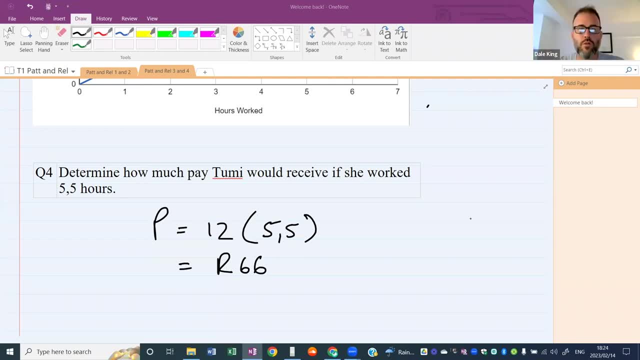 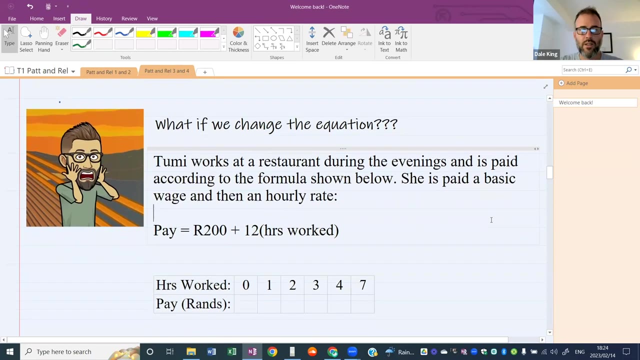 six decimal places. as long as you substitute that number into the formula in the right place and get the correct answer, Okay, let's have a look at what else I have for you. Uh-oh, Oh, no, Dale, what if we change the equation? 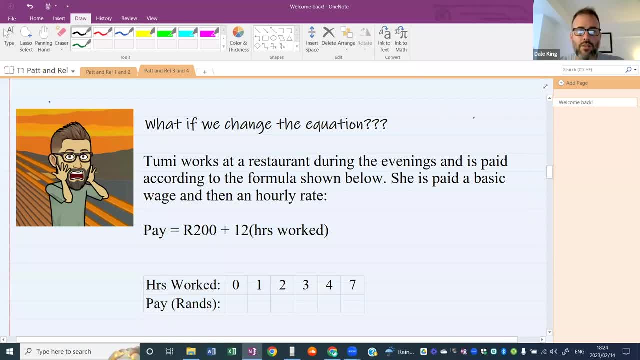 Ay-yi-yi. So same scenario, and now we're going to change the equation. Debbie works at a restaurant during the evenings and is paid according to the formula shown below. She is paid a basic wage. all right, a basic wage and then an hourly rate, okay. 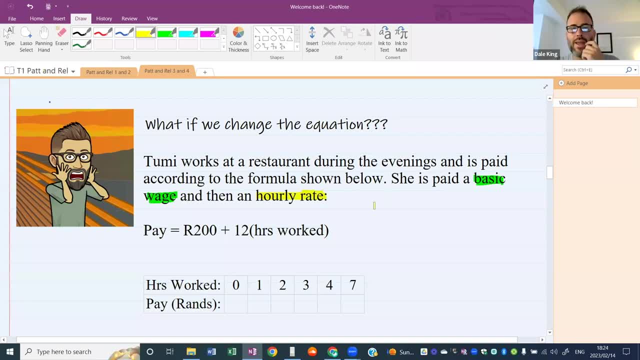 So in the previous scenario we just had an hourly rate. Now we have a basic wage and an hourly rate. So even if Tumi doesn't work any hours, she should still get the basic wage, okay. So even if she just comes to work, 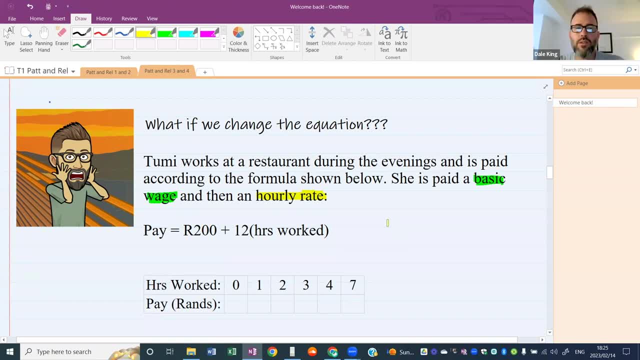 and she doesn't do any work at the restaurant. she should still get a basic wage, which is a much better situation for her. all right, So we're going to fill in this table. I'm going to give you guys like four minutes. 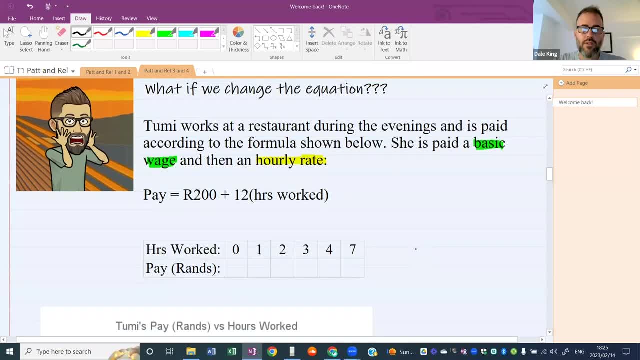 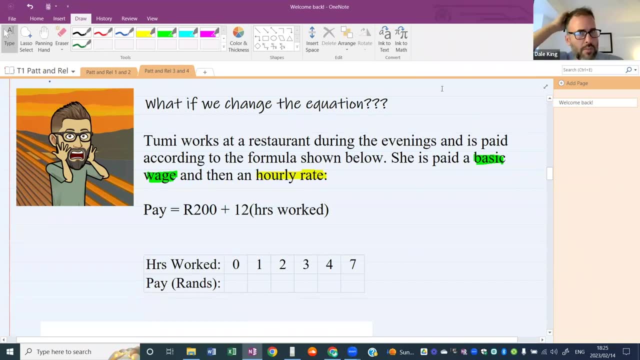 You're going to use that formula, You're going to fill in the table and then I'm going to do it and we're going to check our answers. Okay, you don't have to type into chat if it's too much to type. 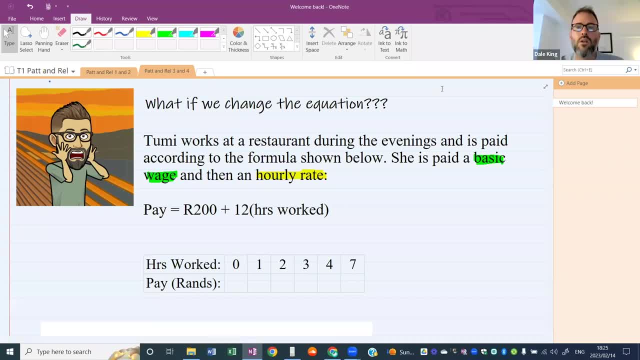 just as long as you have it written down somewhere, as long as you can check your answer with the one that we're going to do here, All right, So we're going to fill in this table. Let's see how it looks. 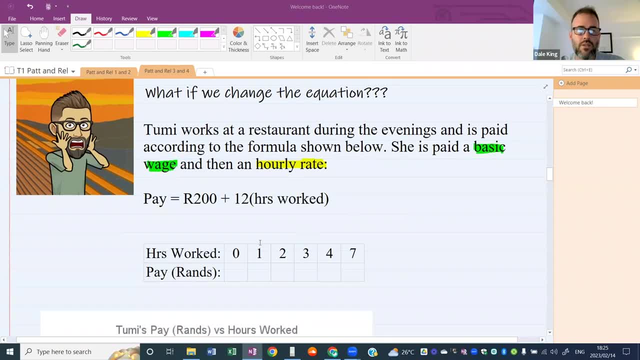 If you want to draw up a little table and then write in the answers underneath, so 0,, 1,, 2,, 3,, 4, and 7, and then just the numbers and underneath, that's fine. I'm going to use the calculator. 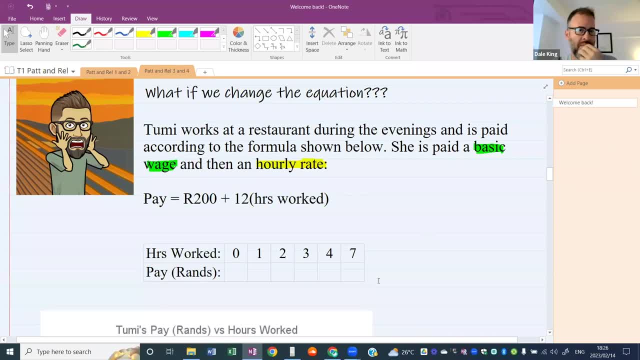 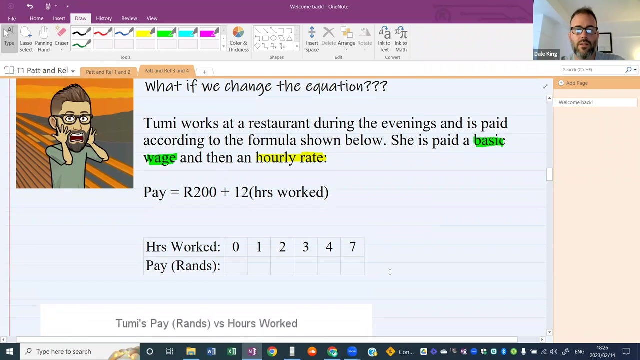 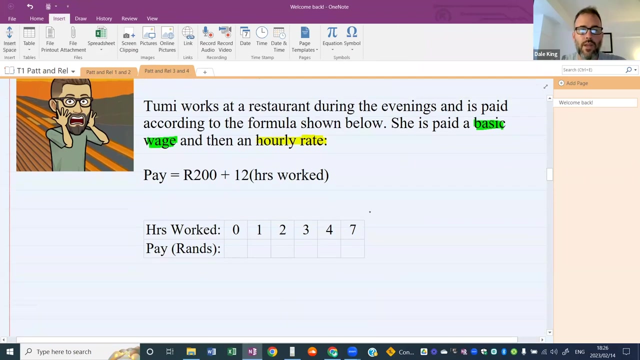 to help me with this one. We'll give you a minute or two and then we'll have a look. All right, I'm sure there are some answers there. I'm going to start doing them and you can check as we go. 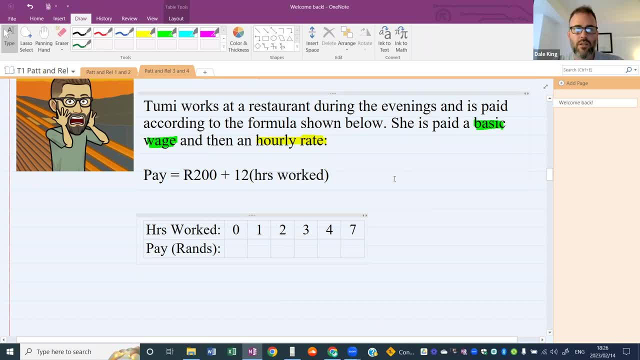 All right, For zero hours. I don't even need to use the calculator for this one, For zero hours worked okay. So we have an hourly rate of 12 grand for every hour, but there were no hours worked. We can't even use that part of the formula. 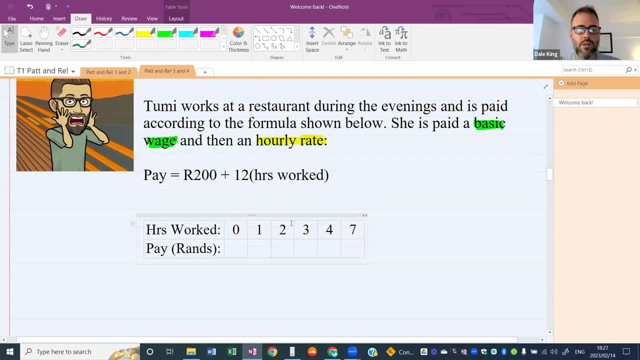 We only have basic wage, okay, So this will be whoopsie. Let's type in some numbers here. so 200.. Let me stretch this table out, All right. So 200.. I'm going to stretch this table out. 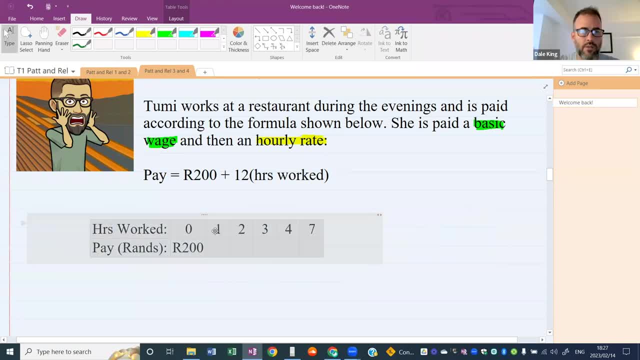 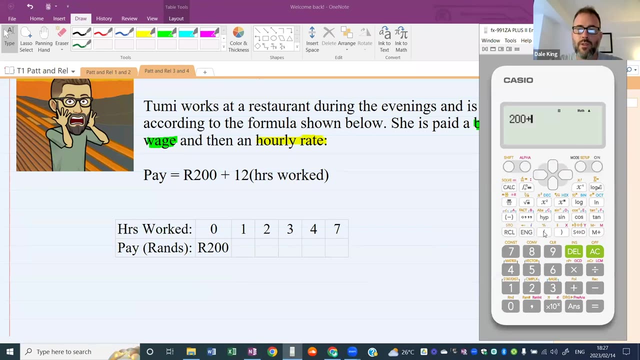 I need as much space as possible. Okay, So we've got 200 grand for zero hours. okay, Now what happens if we have one hour's work? So I'm going to put a formula on my calculator now and I'm going to put a 12 and then a bracket. 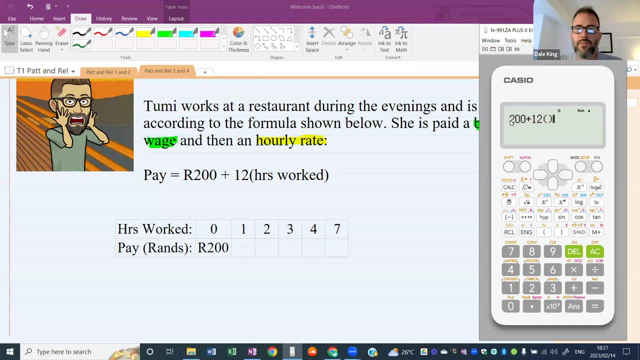 and I'm going to close the bracket. So on the screen there you can see my formula. okay, So what I need to do now is go to that bracket and change the number, So if I put in one there- and press enter. 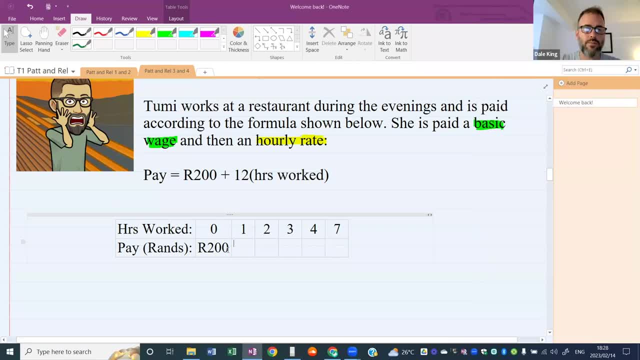 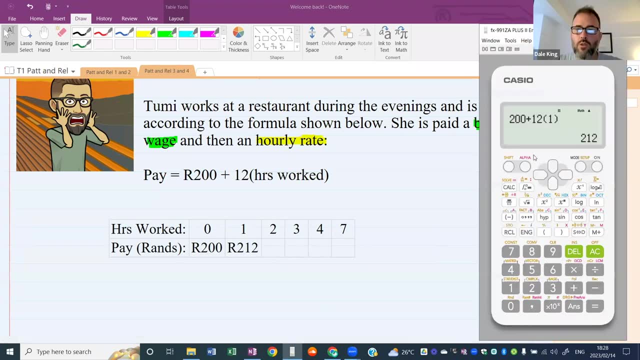 we're going to get 212.. So you've already got that. So 212,. okay, Now I'll go back to my calculator. The formula is still there, So I'm going to go into my formula and just change the one to a two. press enter. 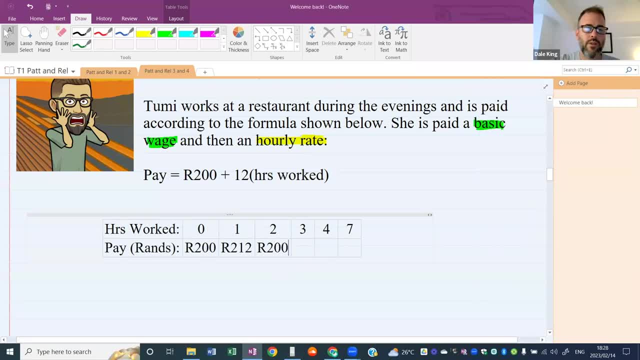 And now we've got 224.. So 224.. Now I'm going to go back into the calculator, change the number to a two. So I'm going to change the number to a two. So I'm going to go back into the calculator. 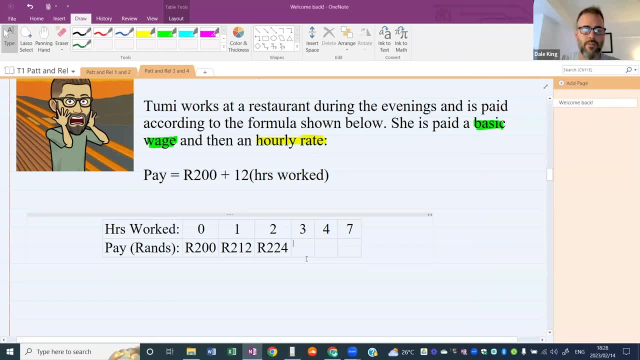 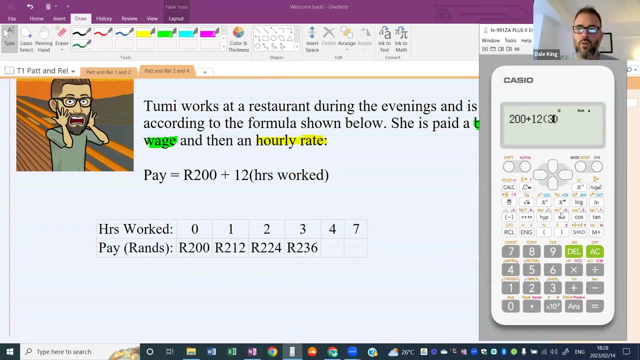 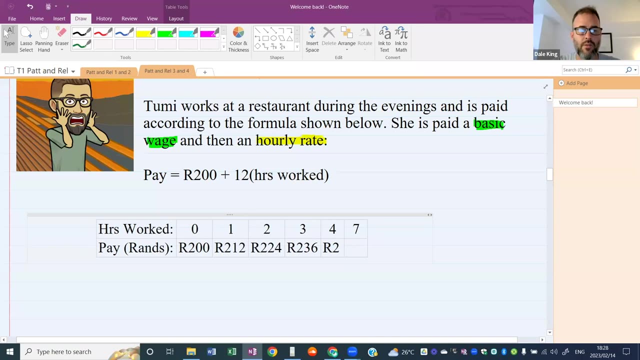 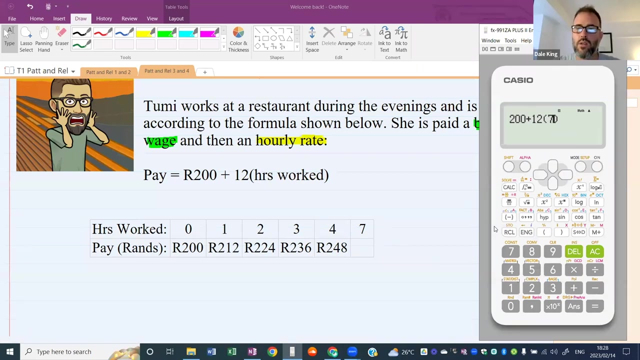 it to three, press enter 236. change the hours mode to a four- enter 248. i mean, it's pretty easy to see what the odds are going to be. i'm going up in multiples of 12 and then here comes the different one. so now i'm going to go in and change it to a 7 and press enter so 284. 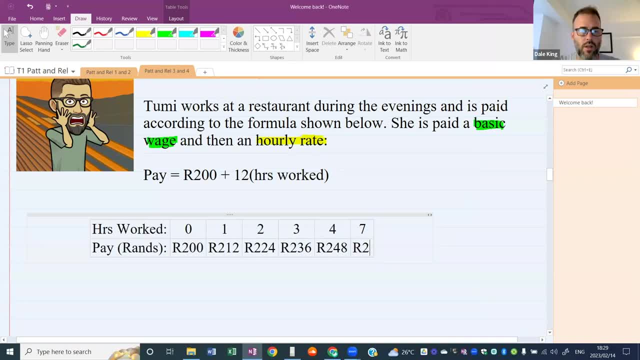 okay, so very similar to our previous answers, but all we have is this: basic wage included now in our answer. all right, now that the words that they use here are basic wage, they can also use, uh, the words a flat rate. okay, almost wrote flat rent. all right, a flat rate. 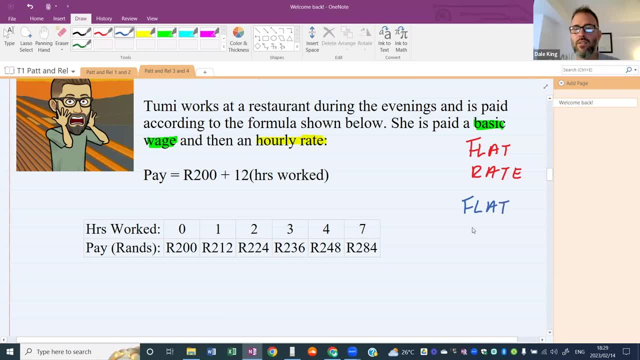 we can also have a flat fee, okay, um, or constant rate or constant fee- so those words are often used to describe this basic wage that i'm talking about here. okay, so all we're doing is taking that basic wage and adding on our house calculation, all right, so these are the values, these are the answers. let's have a look and 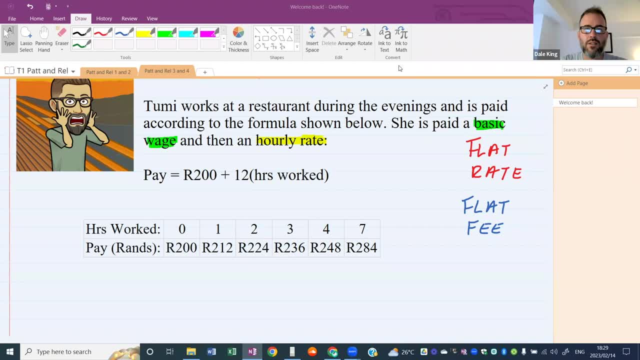 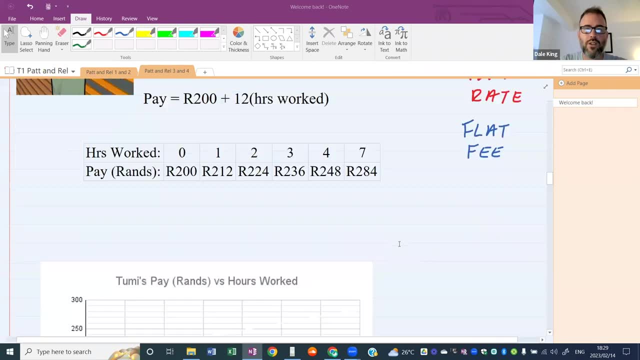 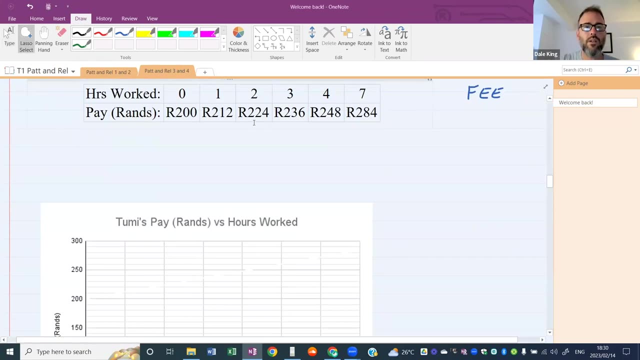 see now what is this going to look like. very good, see you guys too clearly. all right, brilliant answers. well done, well done guys. thanks for doing the hard work. all right, let's see now what this looks like on the graph. i'm going to move this table down a bit. let's see if i can bring it down, so i can. 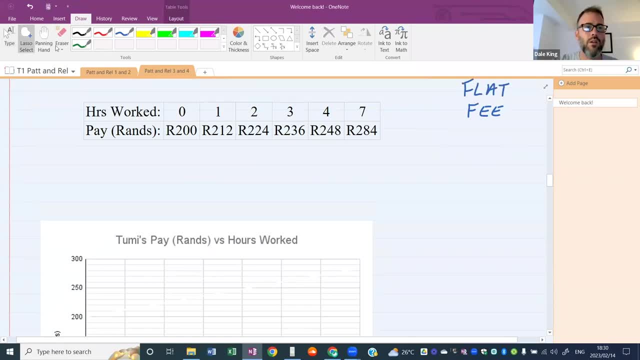 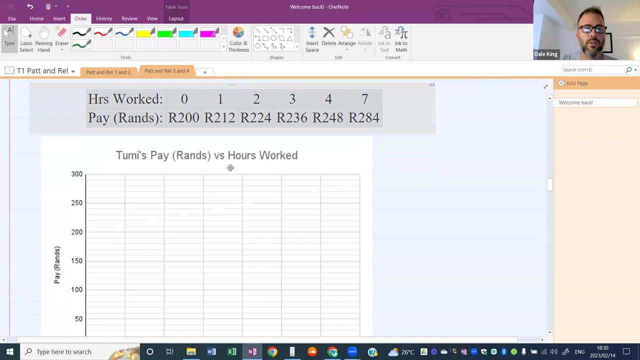 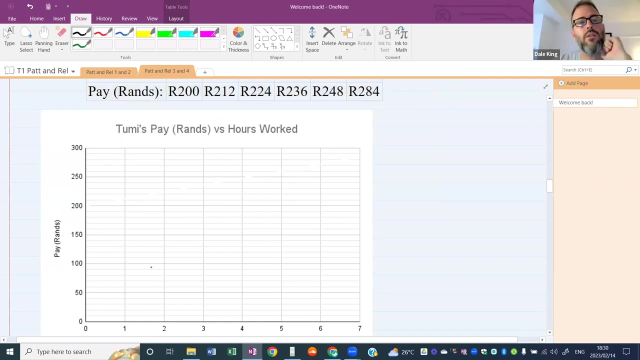 have a look at it while i put stuff into my graph. okay, so here's our table and here's our graph. okay, so for zero hours now, before, for zero hours, we had zero pay, but now there's a basic, there's a basic, uh, basic- wage. so for zero hours even. 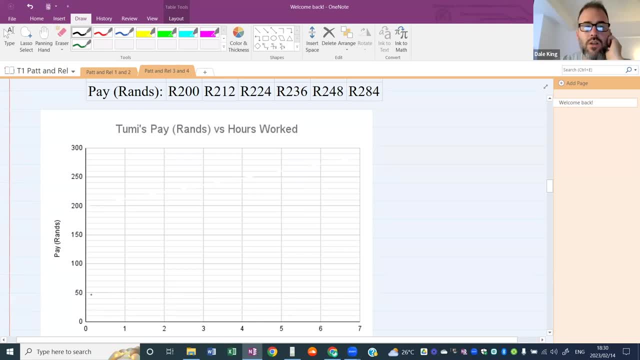 too many, comes in and doesn't do any work. as she gets into the restaurant she's already earned herself 200, so this starts at 200. it doesn't start at zero. okay. at one we've got 212, which is about there's 10. so 12 is about there. 12 is there. at two, we've got two. 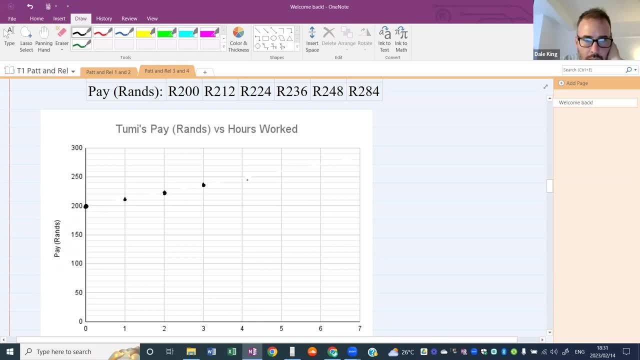 which is about there. at three, we've got three, three, six, which is about there, and four, 248, which is about there. uh, five, we don't have six, we don't have seven, we've got 284, so seven should be 284, that's 280, so it's about there. okay, now again, when we look at our table, this is going up at the: 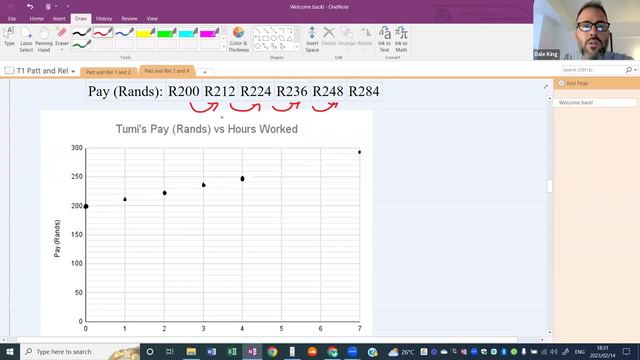 same value every single time, except for the last one. there's a jump of plus 12.. so this tells us it's a constant, increasing graph direct portion, but it's got a basic underlying basic value there. okay, so we're going to start at 200 and try and go through every single dot. 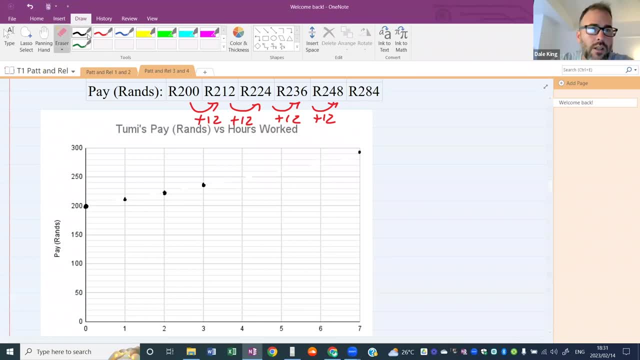 we can see here that one dot was a bit skew. all right, so let's put it back up there and try and go through every single dot. we should still see a straight line. okay, if this table shows us a constant increase of 12, we should still see a straight line. so if your 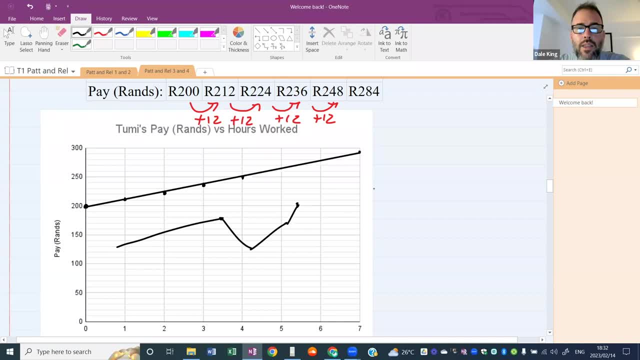 line goes straight and then down and then up and then like that or something like that. there's an error there in your calculation. so you can actually use your graph to check the calculations that you've done in the table. okay, so watch your graph when you draw it. it should be a line if there's a constant increase in the values in the table. 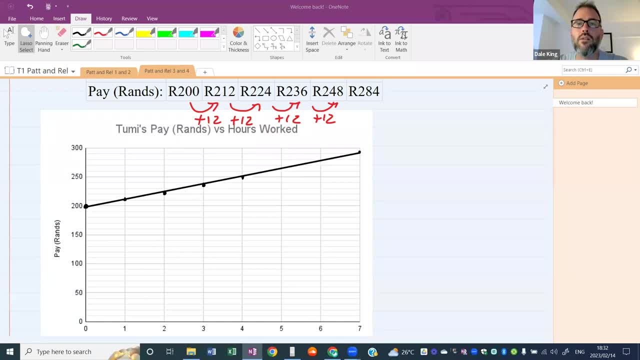 okay, do we have any questions up until now? ah, not direct proportion? yes, there's, it's directly proportional for the hourly rate, but we've got a flat basic in there, so it's not like- not, you're right, not exactly directly proportional. only part of this is directly proportional. all right, anyone got a question? 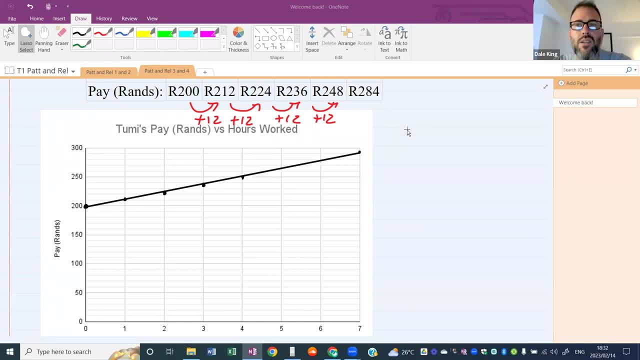 no questions. if there's no questions, then is everyone happy. we're all good, can we move on? i'm gonna give you an example to do now: all right, okay, let's move on then okay, so let's just. i want to recap quickly before i give you this example. 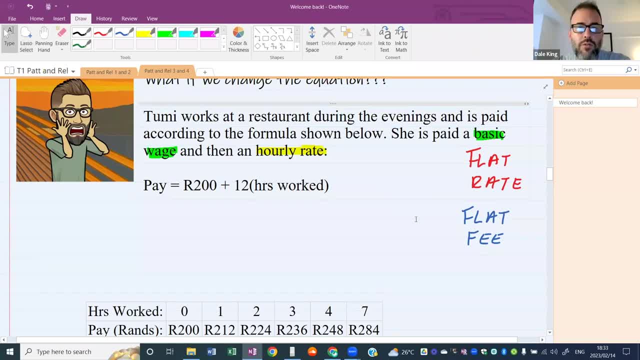 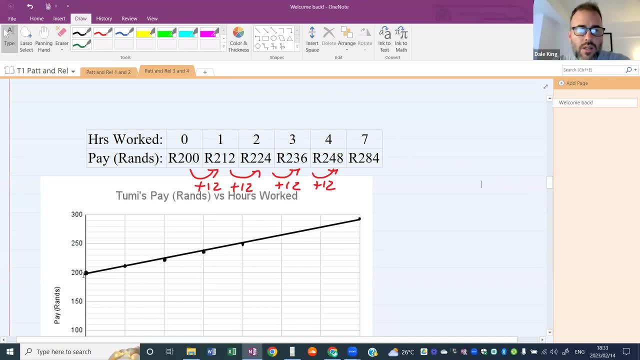 uh, we had a basic wage and a rate in our formula and we still had our formula marketplace rate and we still have this constant increase in our graph. but we have the constant increase starting from 200 because that is the basic uh wage that needs to be added into the formula. okay, 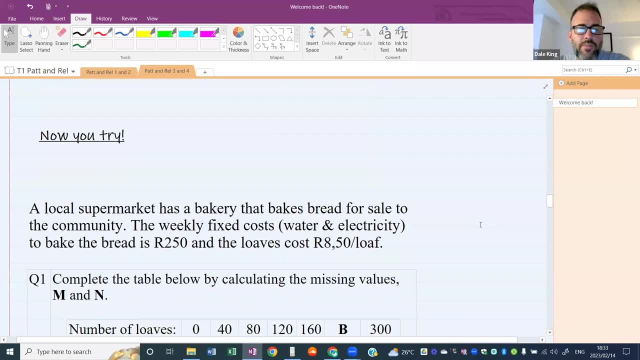 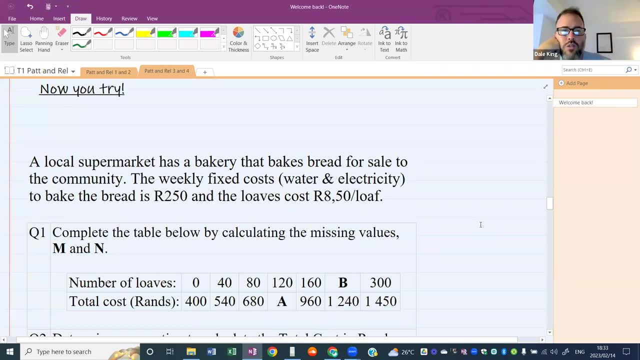 now it's your time to shine right. here's the first part of the question, i think i hope you can see it on the screen. a local supermarket has a bakery that makes bread for sales and community the weekly fixed costs which in our water and electricity to bake bread. 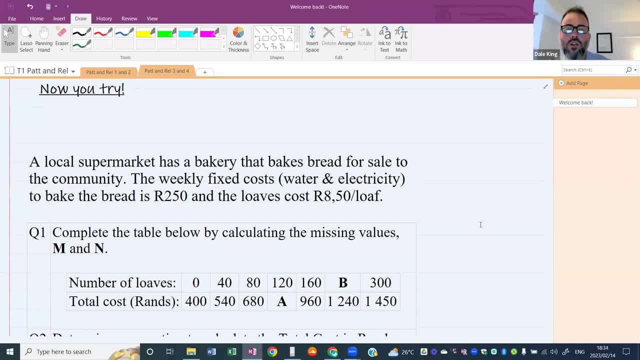 is 250 rand and each loaf costs 850.. all right, so here is a table showing the costs. to break, sorry- to bake loaves of bread. right, this is not pay, this is cost now, and there is a fixed cost. all right, they're using the words fixed cost here and it's 250 rand. 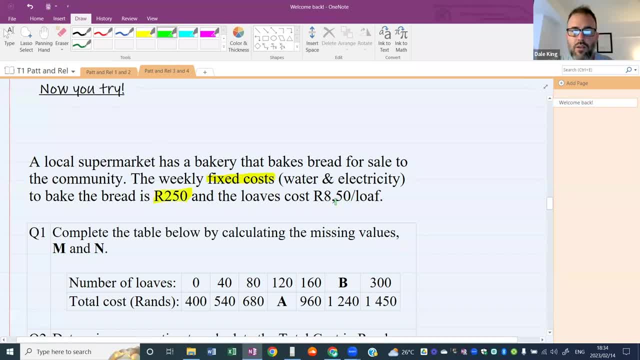 and then we have a rate of 850 per loaf. okay, so there's two parts. that's just like the previous scenario. can you guys please work out? i've got letters m and n, but i'm actually talking about a and b in the table. all right, so we're looking for a and b in the table. 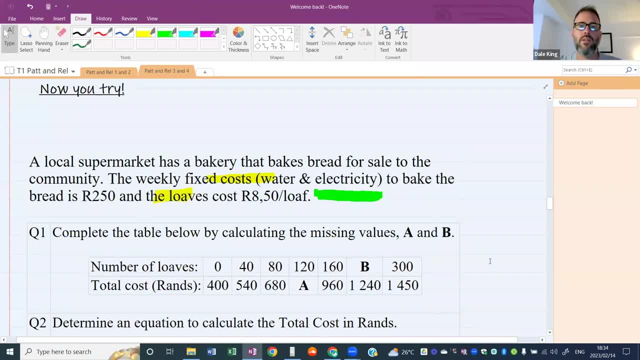 okay, where's g? you can tell me the answers already on the screen. ah, okay, good. no, i was getting worried if guys are reading the answers for question one. oh my goodness, oh my goodness, cattle. all right, it's hot enough. thank you, come on right, we're sweltering in the heat. 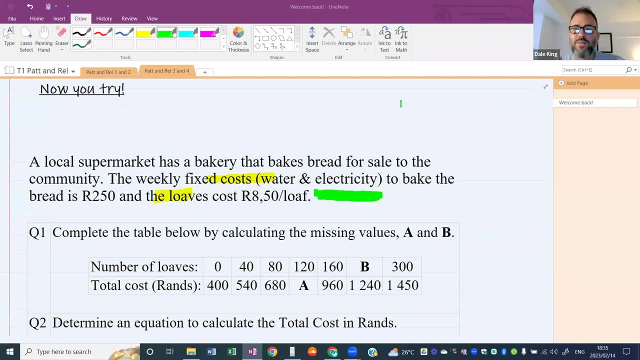 you're bringing fire now to the listen. ah, you see. hey, sonia's fast. yo a is 8, 20.. these guys are fast. i just hope the the um, the quality is good, good speed, good speed and good quality. all right, the answers are flying in. 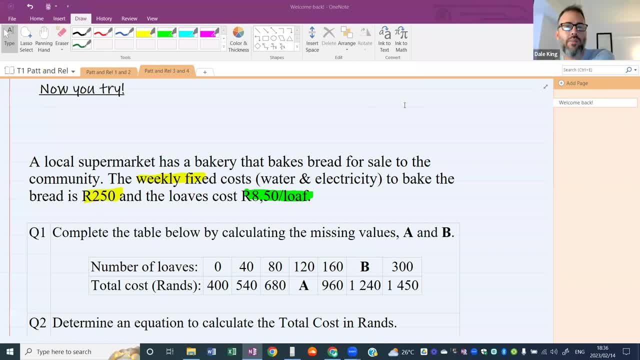 ah, okay the question. the local supermarket has a bakery that makes bread for sale. the weekly costs and the fixed costs specifically to bake bread for in one week is 250 rand and after that it costs 850 for every loaf. so the table shows the weekly costs for. 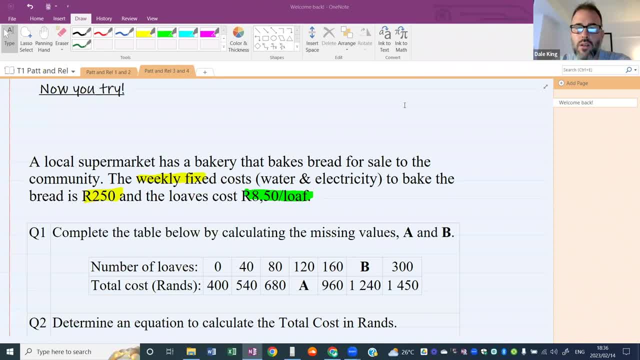 zero loaves all the way up to 300 loaves. okay, so you're trying to fill in the table with different number of loaves in a week and we're just looking for missing letter a and missing letter b. oh, good answers coming in. not that easy. 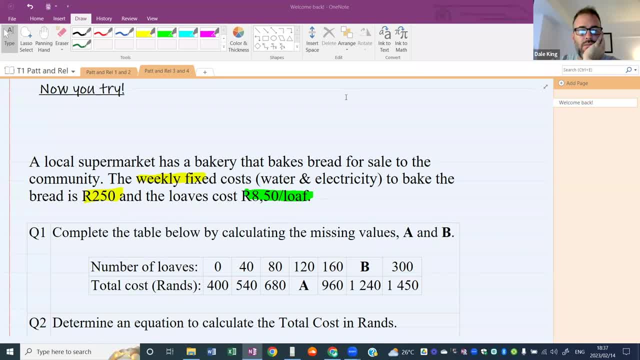 not that easy at all. uh, all right, we'll give it one or two more minutes and then we'll check our answers. all right, the answers are coming in thick and fast. all right, you can see in closely and well, more well, you can see we're using our 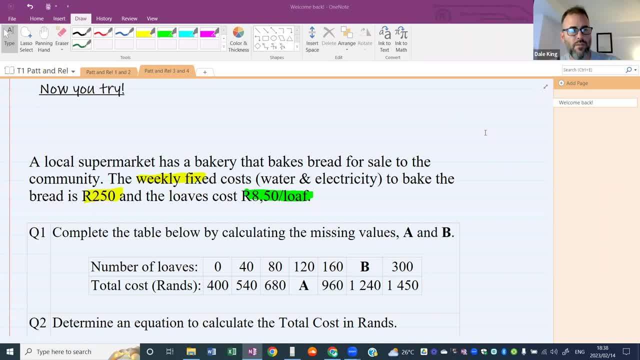 all right, looks like we've got most of the answers in. if you haven't, excuse me, typed your answer to chat, don't worry, as long as it's in front of you or on your calculator or somebody that you can see. so Okay, but it looks like we've got a whole lot of people with answers in. 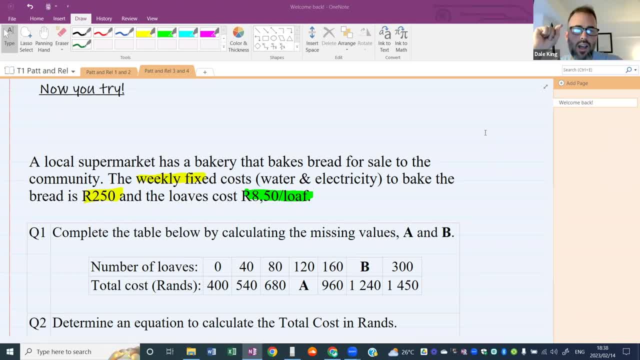 Let's have a look and see how we can do this Now. I'll be very interested to know how many of you used the table to try and figure out your answers, or how many of you used a formula. I'll be very interested to know, because a formula is really easy to use here. 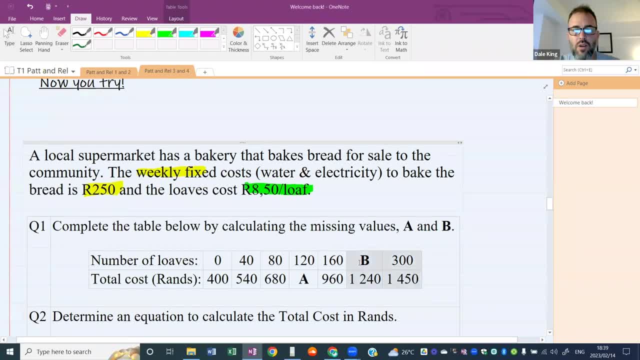 And these last two columns are a little bit different to the first five. Okay, so I'll be very interested to see how you guys did this. I'm sure it would be easier to use the formula. All right, so what I'm going to do is I'm going to build a formula. 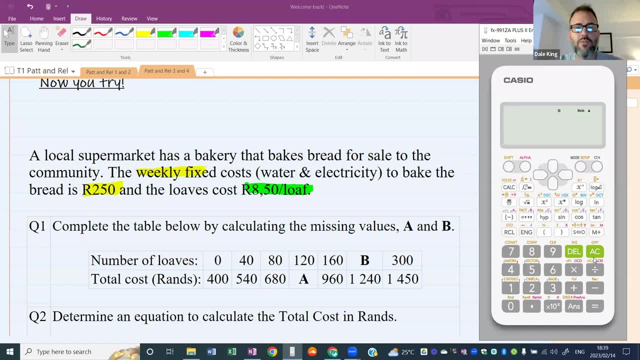 And I'll put it on my calculator And it should give me the same answer over and over again, by just changing the number of loaves. So they say there is a fixed cost, which means no matter how many loaves you bake, you have to pay the fixed costs. 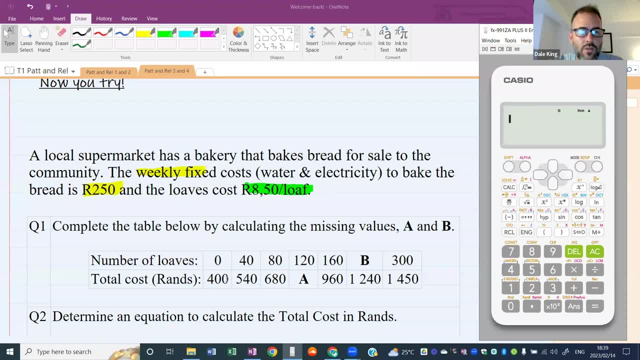 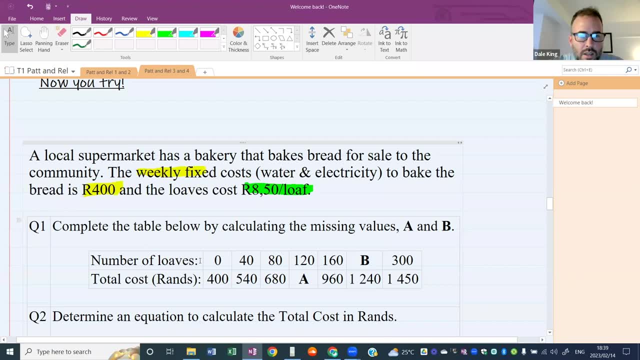 Okay, now there is a mistake in here. The total cost for should be 400,. guys, Look, I'm going to get the stone thrown at me. It should be 400.. Let's check if that's going to work. All right, let's see. 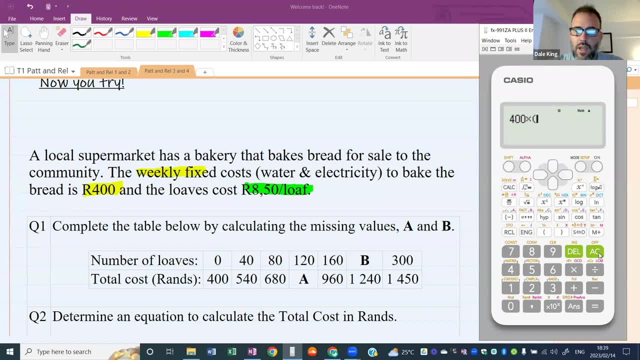 400 plus 8,50 multiplied by 40.. Let's check if this works. Oh, that's wrong. I put times instead of plus. Let's go back. put a plus there: 7,40.. Oh, so this initial one was incorrect. 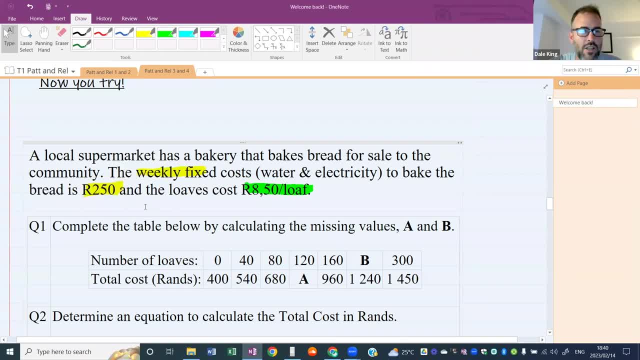 Oh, this poses A fantastic problem. We can actually correct the error with our calculations, So I'm going to delete them all. Okay, there must be an error in the calculation, All right, I'm going to delete them all. Which one was A? 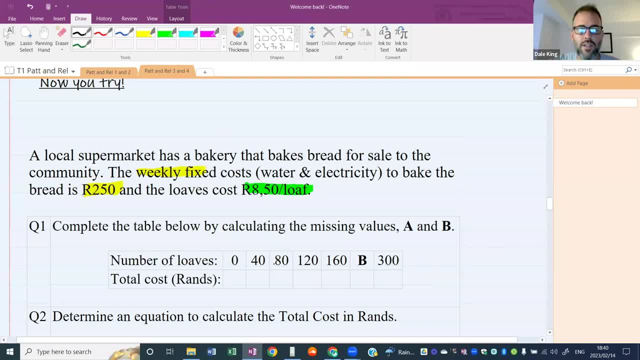 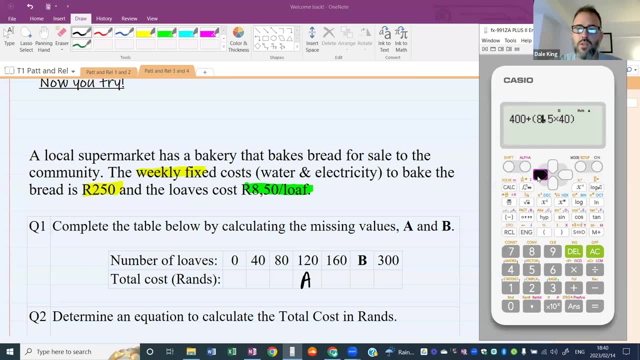 120.. Okay, So A was over here, Let's see. All right, So this is the formula that we have to use. I'm going to go back to the 250 that was originally there. This is the formula that we have to use. 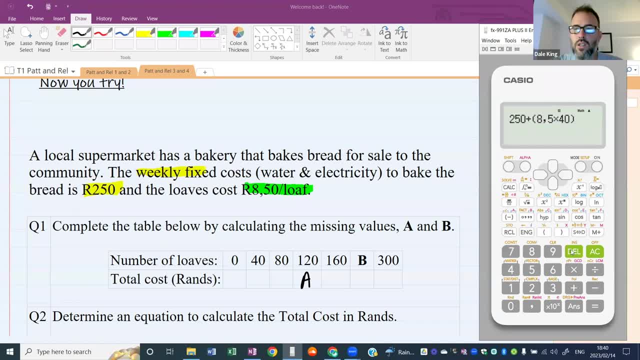 This poses a fantastic opportunity. We're going to put in all the information. All right, So 8,50 per loaf and 2,50 as a fixed weekly cost, Let's see what we can get. Okay, so if we bake, 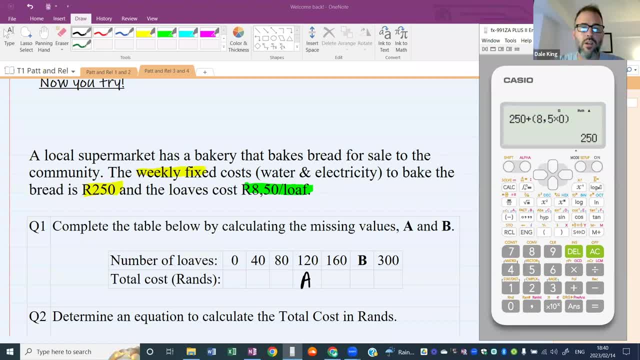 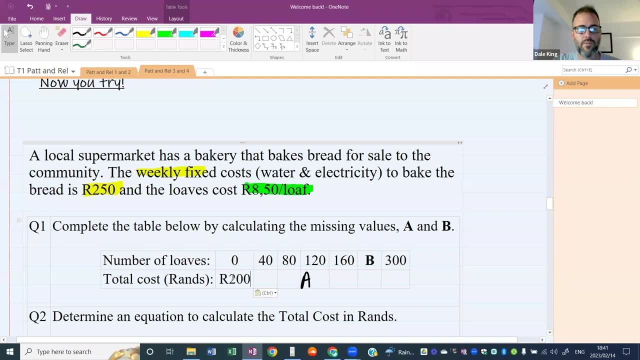 Let's in fact do the first one, which is zero. So put in zero there, We should get 250.. Okay, So I'm going to type them in as we go: 250.. And then go back to the calculator. What if? 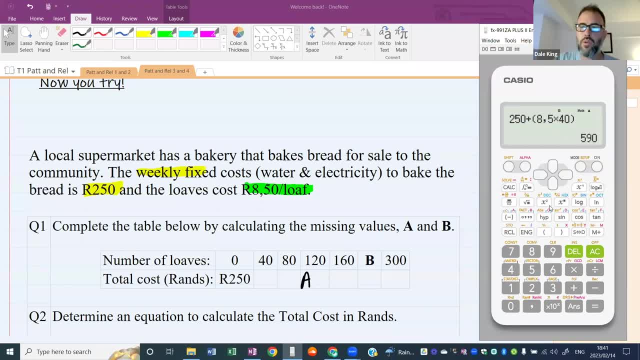 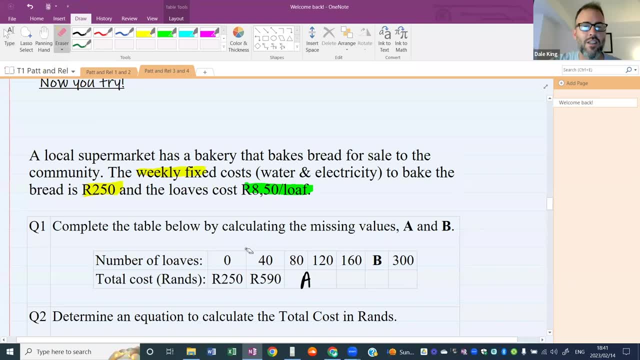 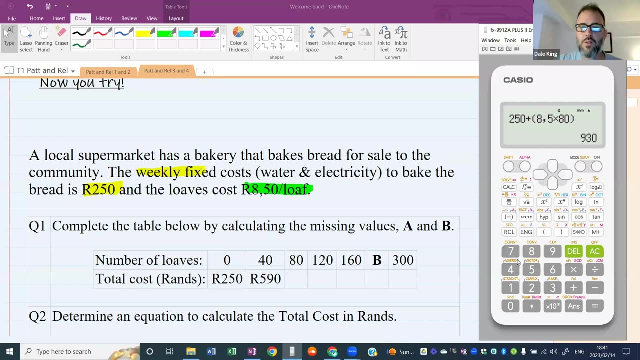 If we put in a 40 there- let's quickly fill this in and press enter- We should get 590.. I'm very excited to see what the answers are going to be Very excited. Okay For 80.. Let's change the 42 and 80 and see what we get. 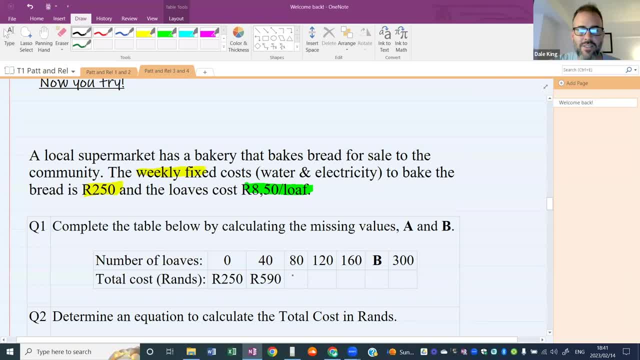 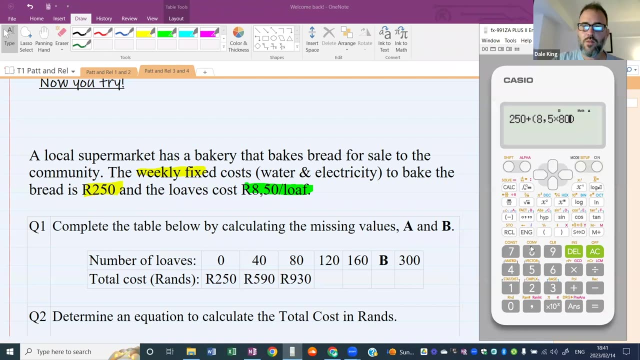 930.. Oh, I wonder if people are worrying about the answers. now, 930.. Okay, What if we have 120?? Now, 120 was A. All right, 120 was A, So let's put in 120. using our formula from the question, we should get 1,270. 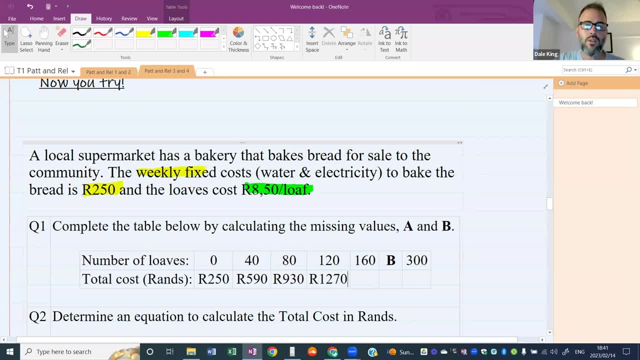 That is huge: 1,270.. All right guys, I'm in the wrong business. I should be breaking, breaking, breaking. I feel like you feel like breaking things today. Yeah, I do, Yeah, Okay, So breaking bread. 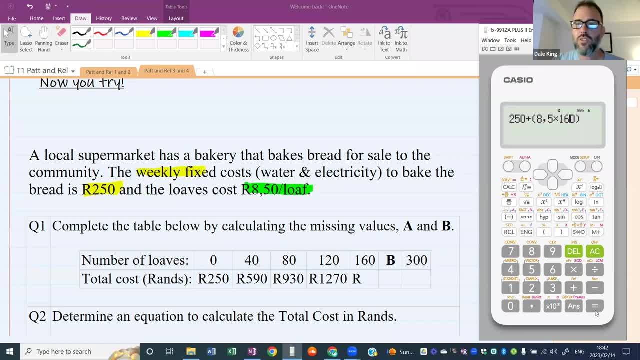 That's what people do actually at dinner time. They break the bread. It's a traditional thing. All right, One six, one zero. All right, So one six one zero, And B was one that you had to get. 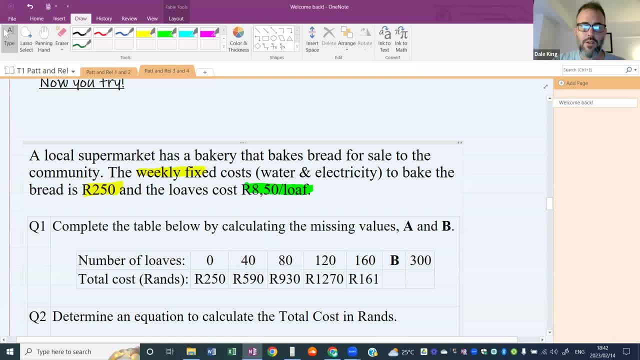 Okay, So I am going to come back to B, But let's go back to 300 for now. Let's put in 300.. And 2,800.. Now this really poses a lot of questions, Okay, So let's go back to B. 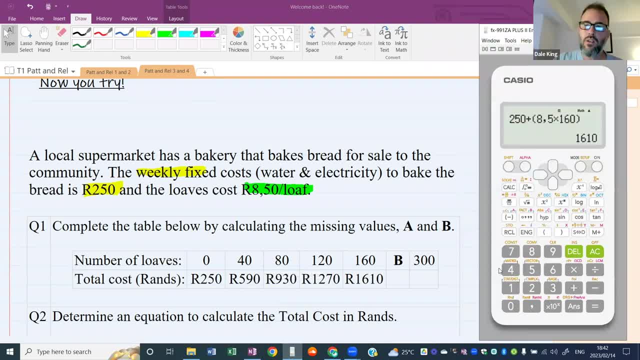 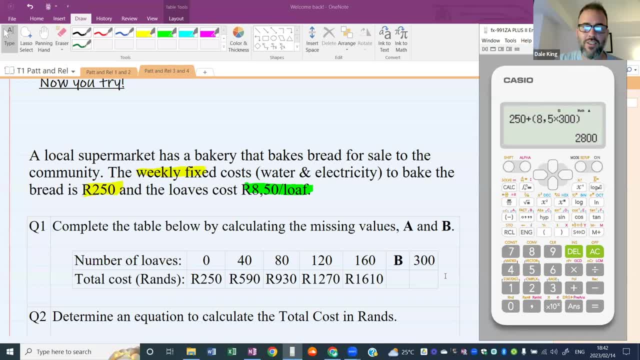 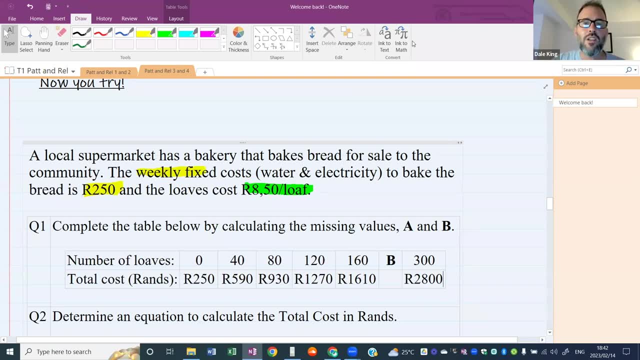 Let's go back to B And 2,800.. Now this really poses a very interesting scenario, Because if I go back to the answers, if I go back to the answers, yeah, you see 820 and 240. 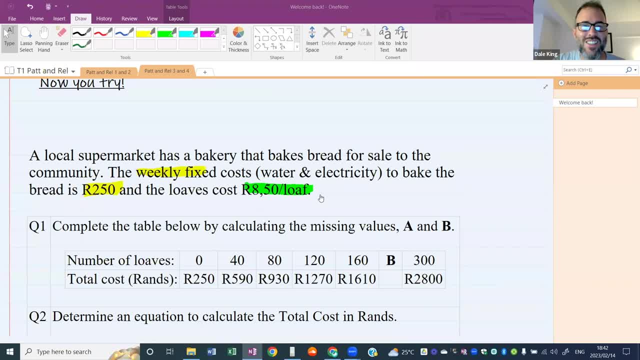 Now I think the people who are getting 820 and 240 didn't create a formula And I think they looked at the difference between the numbers in the table. then try to infer from that, okay, the numbers. there was a mistake in the in the numbers in the table. 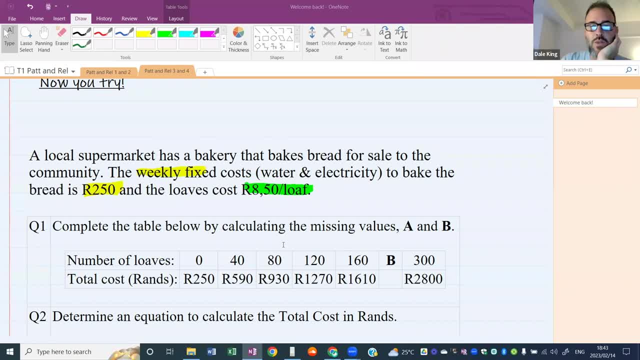 so the formula and the numbers in the table weren't correlated. so if we corrected this and remove all the numbers in the table and just use the formula, these are the answers that we should get. you have to agree with me. so i think what you guys are doing is using the table to 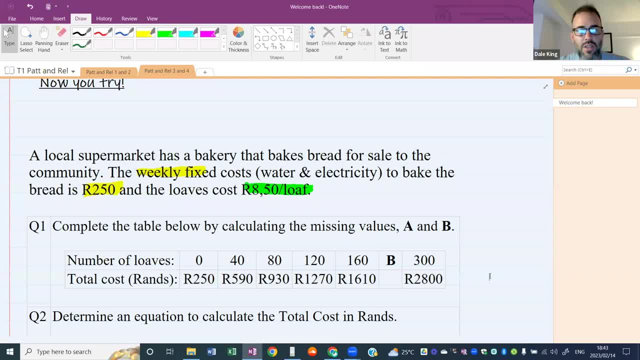 help you get your answers, which can be tricky because sometimes they won't make the first five or four numbers consecutive. they might make them totally different. they could put 130 there and they could put um 50 here and make them absolutely different, and you won't be able to find a consecutive pattern okay, so you're going to have to rely. 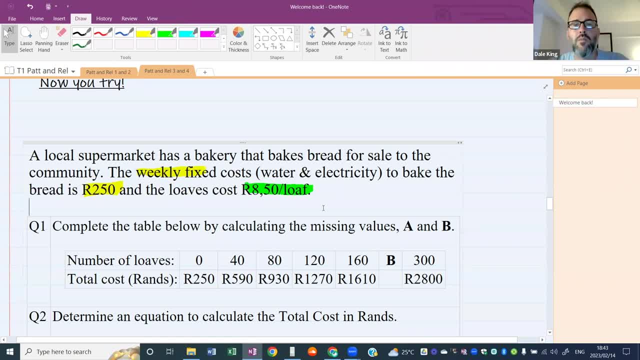 on the formula. in fact, that's why i said: i hope you guys are using a formula here, because it's the safest way to solve this problem. all right, so 120 was 1270 and let's go back down to b. uh, to find b, we actually need a value, okay. so what i'm going to do is i'm going to create a value. 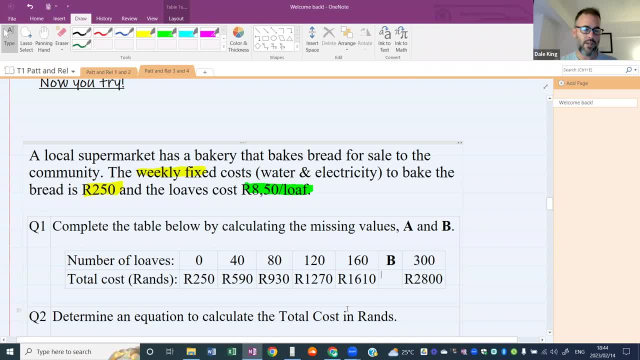 how do i do this in secret? ah, i'll do a secret over here. i'm going to put a value in and then you guys are going to tell me what the value is. all right, let me find a secret value, okay, so and oh, i've got a value. 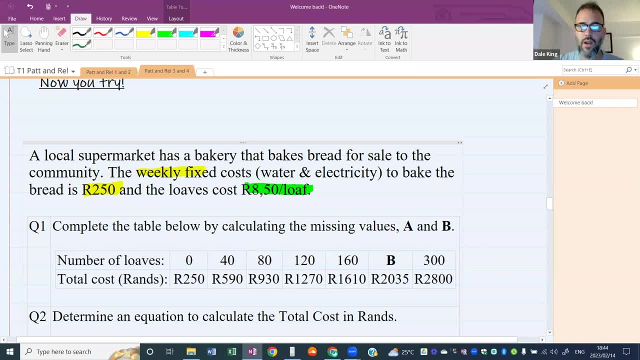 of 2035- 2035. all right, let's see if you can get b's value from 2035. everybody is saying that they're a little bit confused. i'm going to go over it again. i just want to see if anyone can take this. 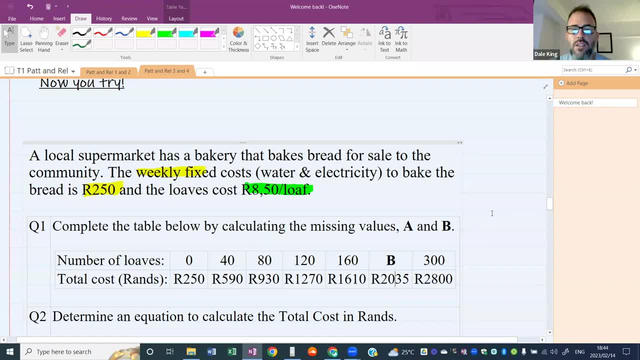 total cost and use a formula to get b's value, and then i'll explain it one more time. it is a bit more challenging, let's see. i'm sure someone there can get a value for b, and then i'll go over this one more time. there was a guy on last week. his name was pabalo. 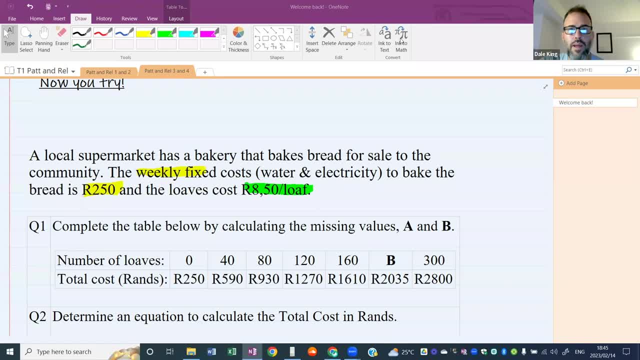 and i think pabalo managed to work backwards in the formula to get an answer similar to this: wow, and he's not here today. he's not yet they are. they're asking: how did they get um the 250.. oh, that's the fixed cost. 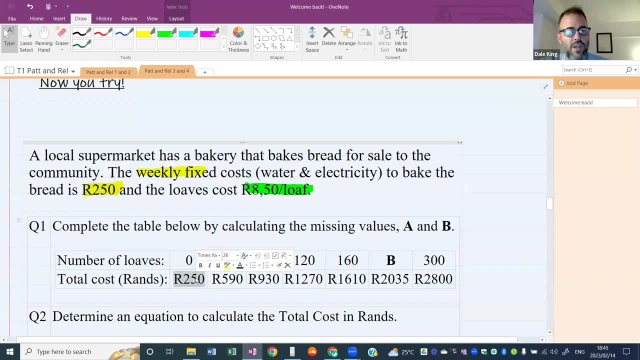 in the question there's a fixed cost of 250, so the original table had 400 in here at that starting point, i think. and what guys did was they worked from that 400 table onwards to get their values. so those, if you ignore the question and you go straight to the table and try to use the 400. 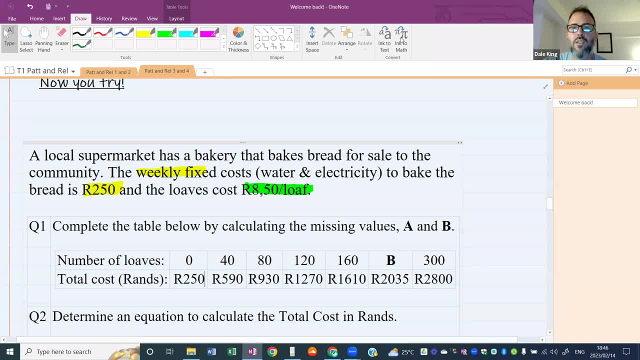 then it gives you different answers. uh, that's not your medicine. all right, let's go back to the original question and see. if you can't find it again, let's go back to the original question. i think that about it will pop up there. ah, there they go. all right, so this was the original scenario. so we had the. 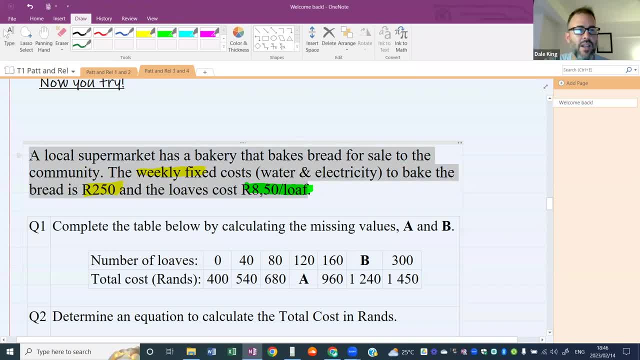 texture with some values in. okay, and i said that we have a weekly fixed cost of 250 and lowest cost 840.. but if you look at the first value in the table, it's 400, which means that this fixed cost and this 400 are different, which should be different. so if left to your own devices, 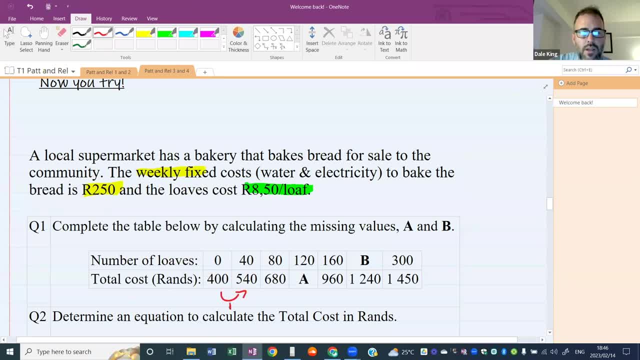 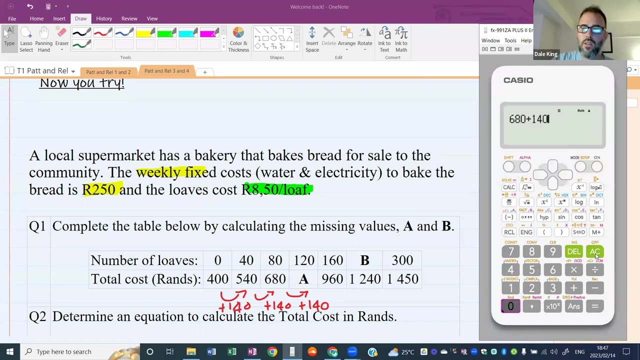 what you guys started doing was you started saying: well, there's a increase of 140 every single time, and then you use that to help you get a. so 680 plus the 140, 680 plus 140 is 820.. that's why guys are getting answers for a of 820. okay, because you've been 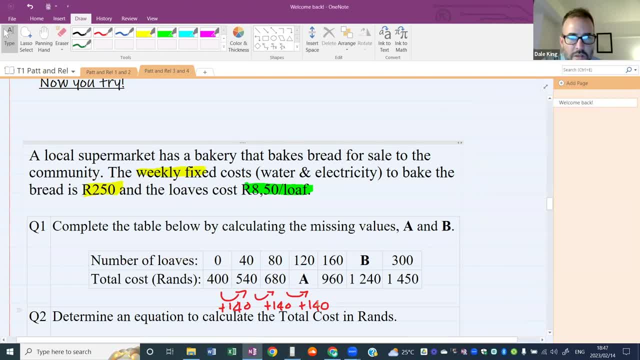 using the, the rule of there's a constant difference every time. to jump to the answer, are you using the table? you definitely didn't use a formula for that one. okay, so you use the values in the tab, which is enough, which is the correct way of doing it. okay, but there's a mistake in these values. all right, so we had to change the. 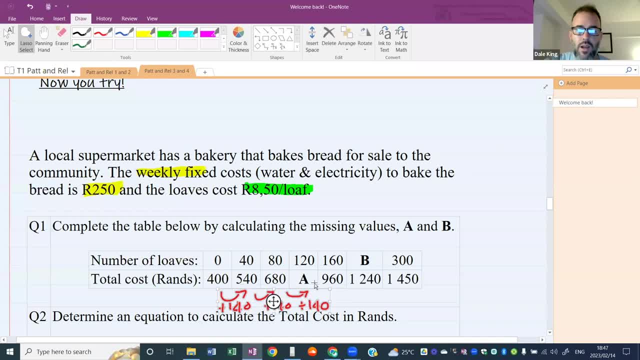 values in the table, and we don't do it by looking at consecutive numbers. we have to use the formula. all right, so what i'll do is i'll show you again how i did it. i said: ah, these numbers are not correct, let us remove them and let's recalculate them, okay. 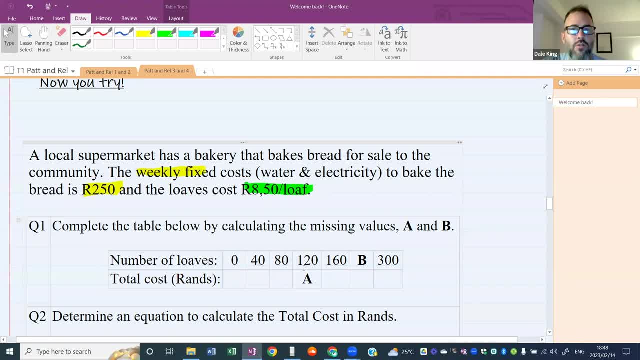 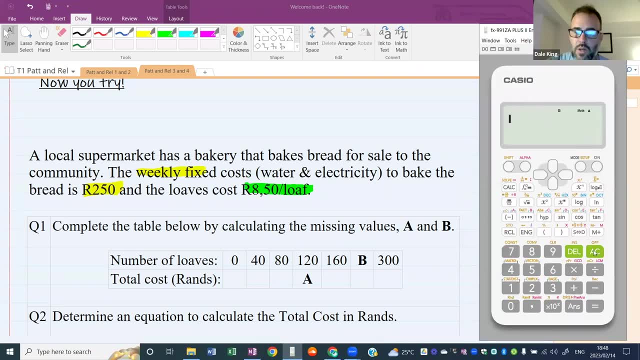 all right. so let me do this again. so we do that here. you can see we have right. here is the formula. okay, so if you take this table and youächlich for 1 second and you're just playing the table and then you choose this one, okay, so now you can't find values for any of these. 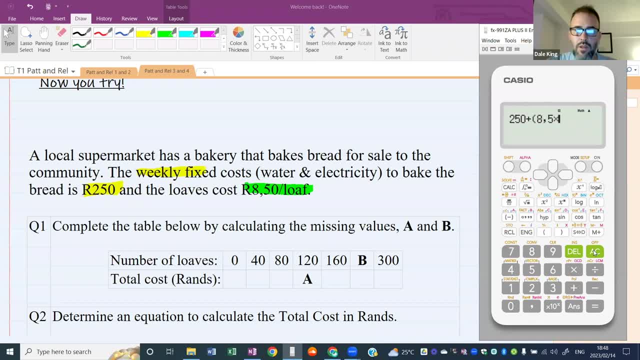 unless you have a formula which is the best way to solve this problem. all right, so we're going to. for the first one, we have zero lobes. okay, i just got it in brackets there because in my brain i like to do certain parts first and i use brackets there. but the calculator, even if the brackets, 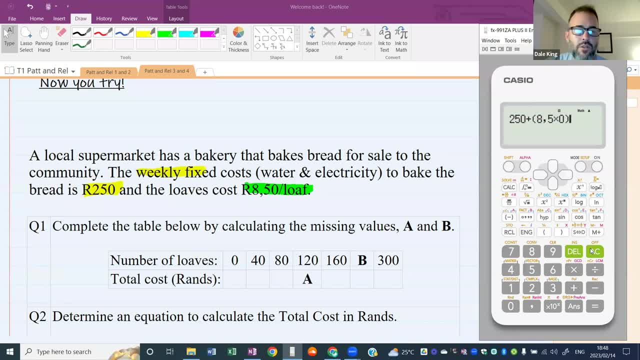 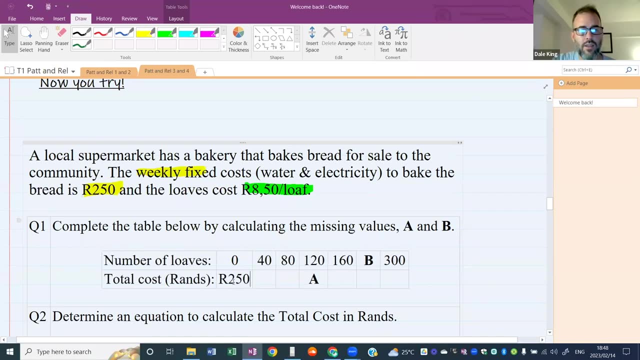 went, they would would do that in 50 times zero first. all right, so now i'm going to say if, using this formula, what do i give? i have zero lobes and the answer is 250, right, so i'm going to put the value back in there: 250. so we see here, this is correct, because the fixed value is 250 and 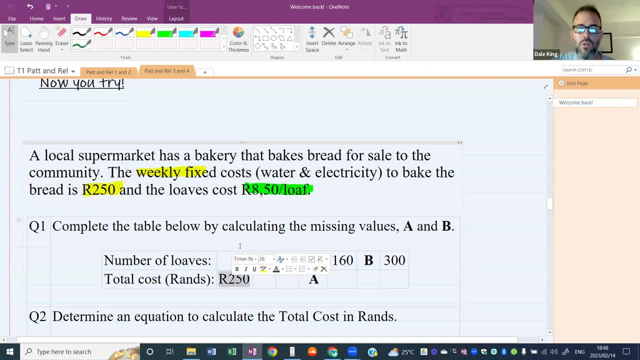 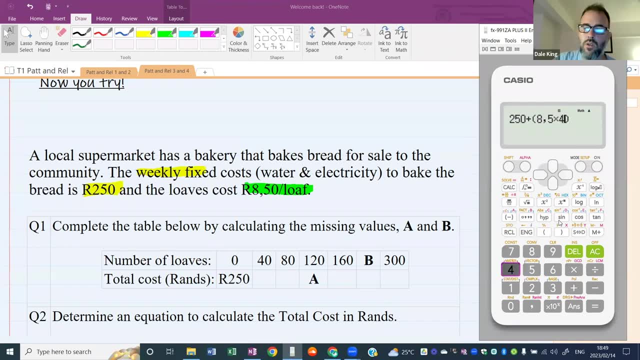 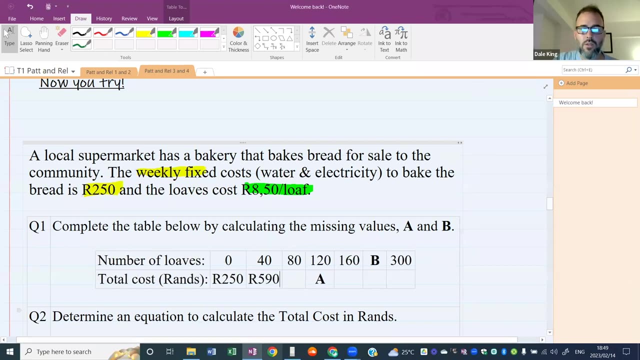 without cooking any loaves or baking any loaves, we should still have 250 rand as a cost. all right, now i'm just going to change the formula and change our number of loaves to 40 to get 590, and then i'm going to do a change to 80 and that gives us 930. these are big values now. 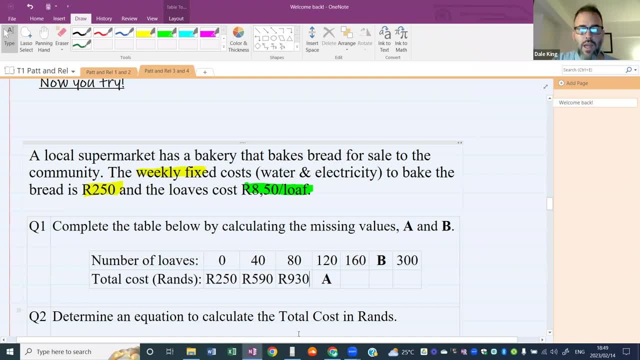 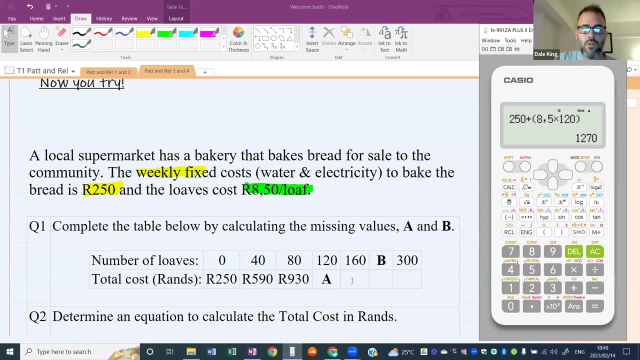 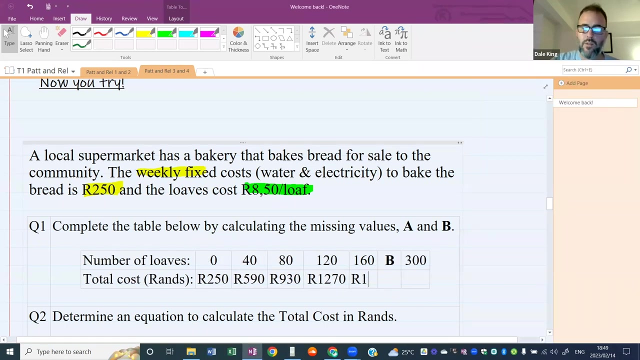 and for a. we can work that one out straight from the formula, change it to 120, so we get 1270, 1270, and for 160 it's 1610, 1610 b. i'm going to leave out 300, we can do. 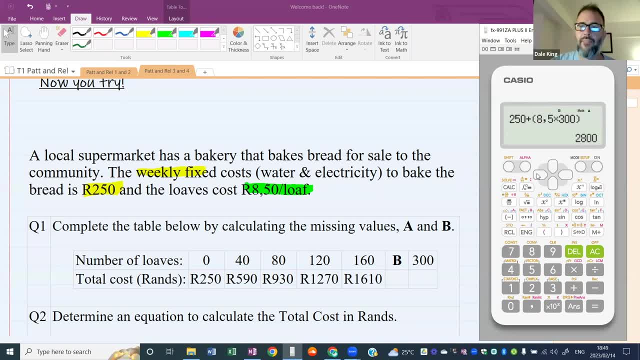 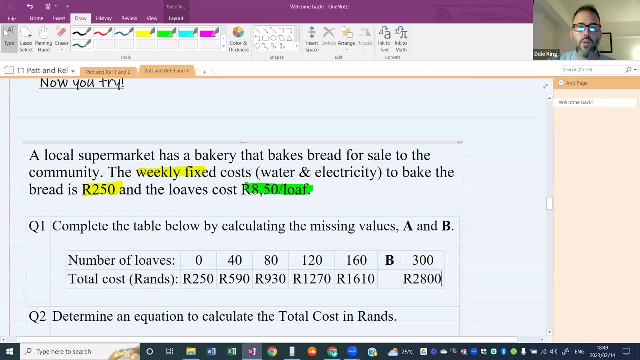 000 and that's 2 800.. all right, the question is: can you find b? and i put in a value over here. if the rand value is 2035, ah, there we go and then go on. that's it. that's the form you need to use, okay. 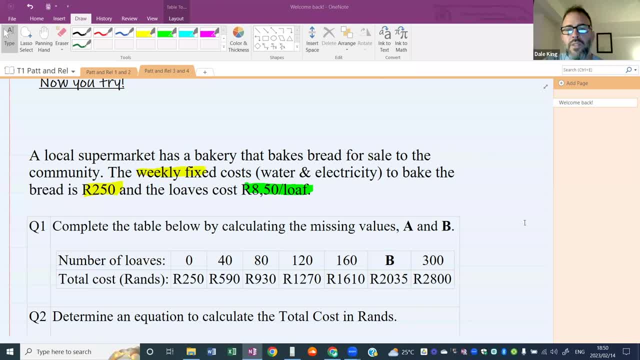 yes, i'm still fighting with the Macbook for not allowing me to film during the game. all, all the lessons ending at seven. we're almost done right, so let's see if this is we can do this last question and then i'll show you the equation. i'll just write it out underneath, but let's. 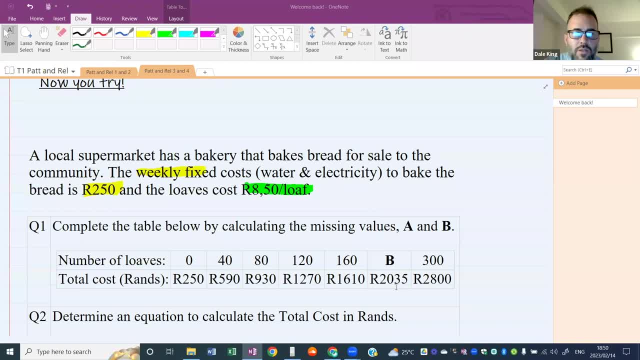 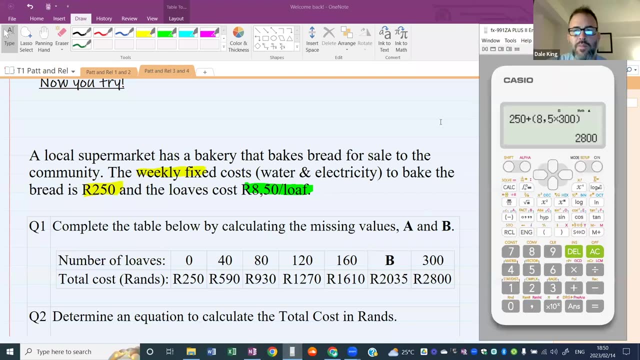 see if you can find out b's value if you have 2035 red as a cost. thank you, all right, 2035 as a cost. can you work backwards? here's a formula on my calculator. if you want to work backwards, all right, but just remember that we don't know what that value is. okay. 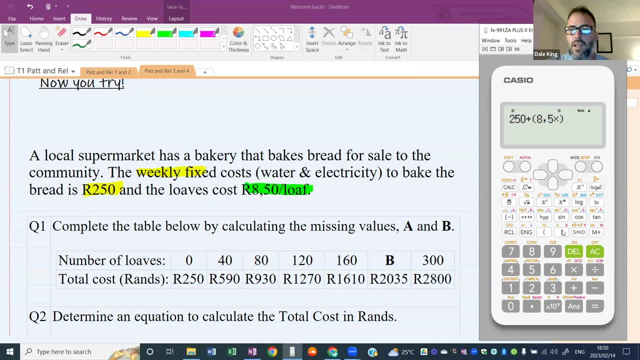 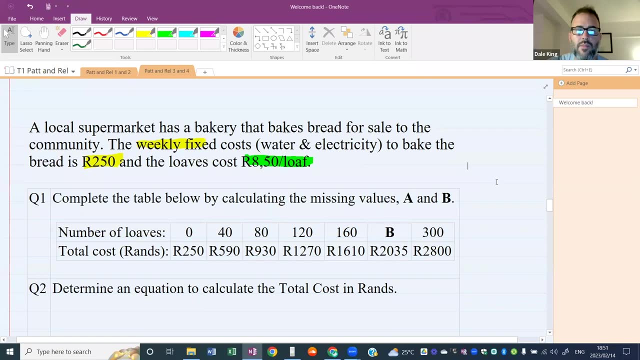 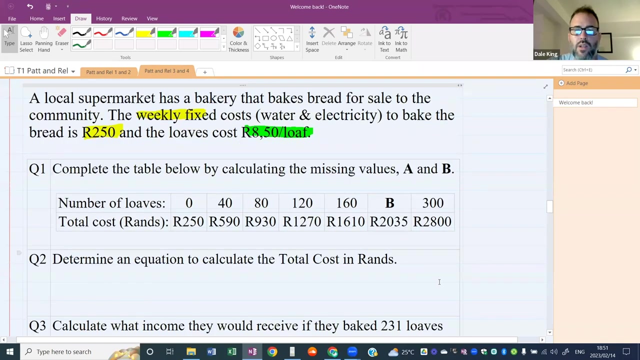 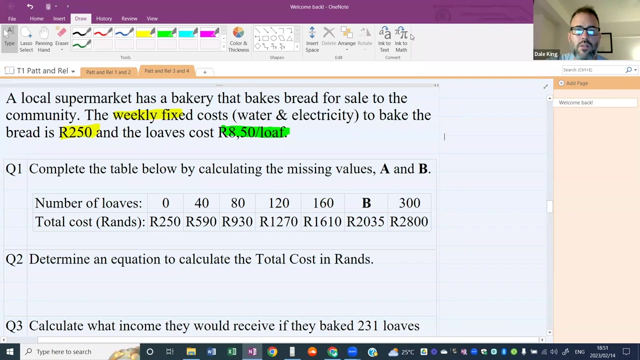 you can think of it as a missing variable like x. all right, what is that x value if the cost is 2035, right? so let's see if we can find out b's value in the answer here. okay, anyone, let's, let's, let's show this to you guys. we'll work backwards. oh, do we have an answer? 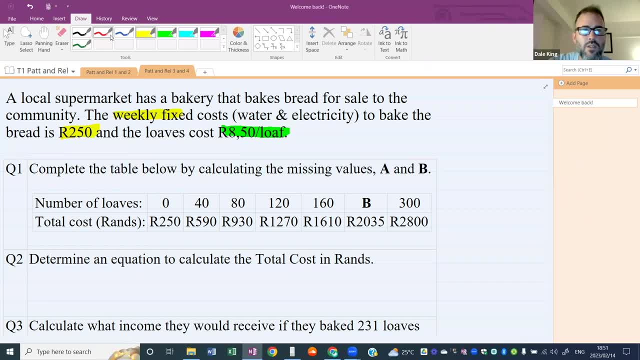 and we wanna- yes, we are. we are adding 40. there is a constant difference here. yes, there is a constant difference here, up until there are totally different. so we can't use constant differences to find these last two. we're going to have to use a formula. so i want you guys to try and learn how to use a formula to find these. 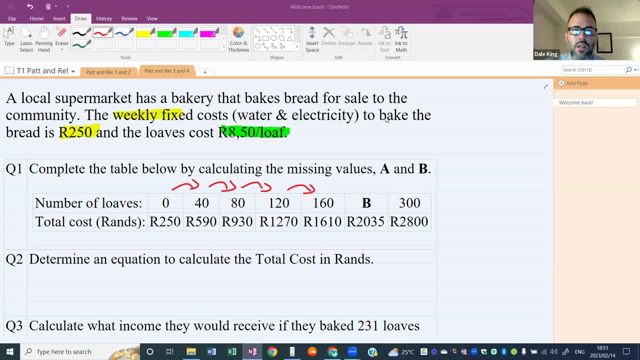 uh, all right, we've got an answer there of 210 from christy. okay, i'll give you one more minute and see if anyone else can try to figure out 210 from ave. good guys are using the formula now, which is fantastic. all right, let's check if these two guys are right. i'm sure they're more, but let's see if they're. 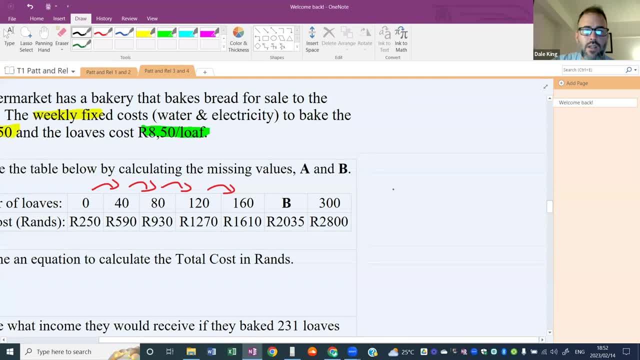 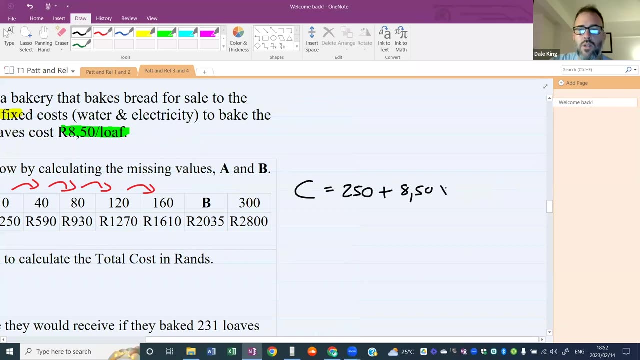 correct, okay, so the formula we're going to use is: i'll use c for costs, okay, and we need 250 rand plus we need 850 times the lobes. all right, i'm going to say l for lows. i'll put that in a bracket because i really want to do this one and i want to add another one to the box. 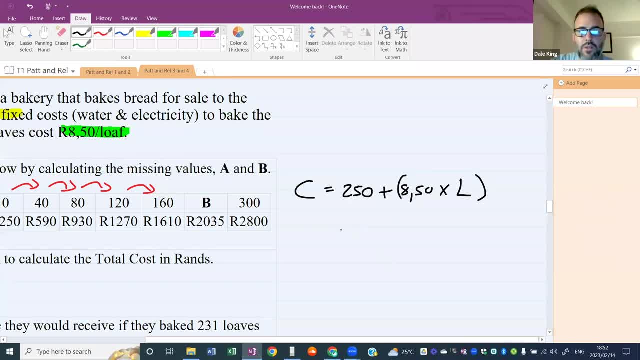 do that one first on my calculator, but the calculator will do that first anyway. with that part there's bod mass says you're going to do multiplication first. okay, so the cost is 250 rand plus 8 rand, 54 times the number of loaves that we have now. we don't have the number of. 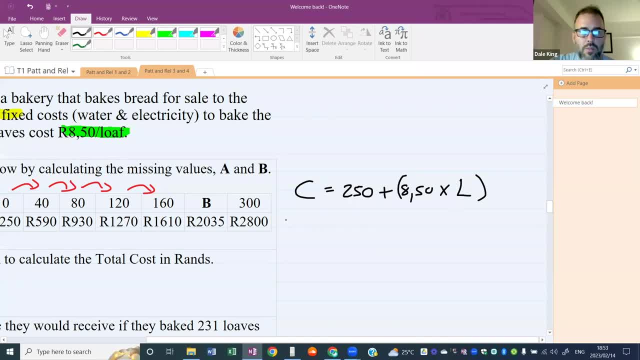 loaves. we're trying to find the number of loaves so we have a cost. so i'm going to put that in on this side. so 2035 is my cost, okay, and this is 250 plus 8 rand, 50 times the number of loaves and i. 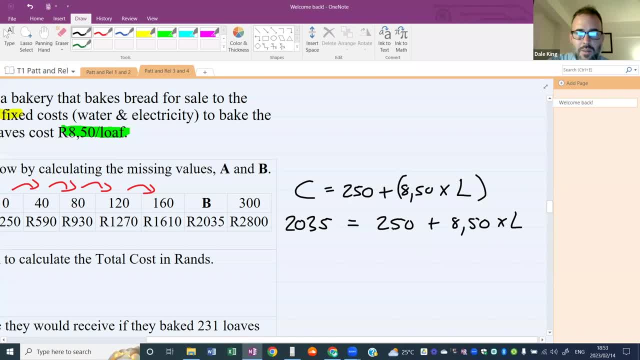 want to find the number of loaves. all right, so the first thing i'm going to do is i'm going to get rid of this 250 rand. i'm going to take it away from the right side of the equation and move it to the left. so we're going to first subtract. 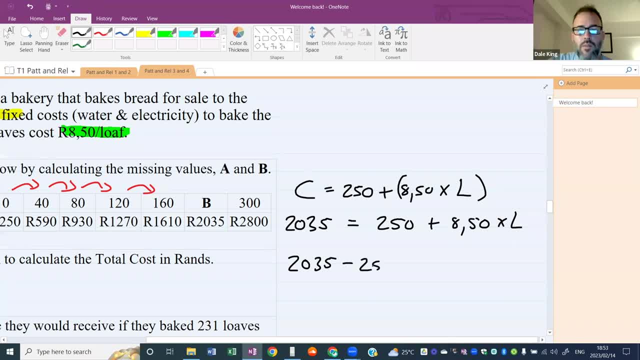 250 from our cost and this will give us 8 rand, 50 times the number of loaves. all right, so let me do that on the calculator. so 2035 minus 250, that's 1785. so if we remove the cost, the fixed cost, we get 1785. 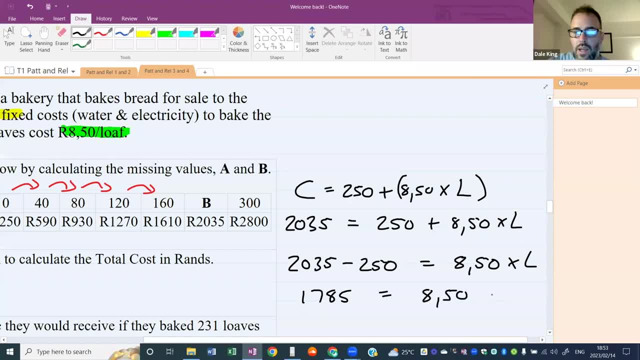 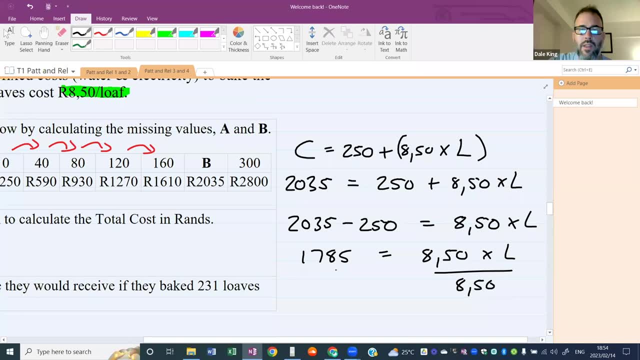 for the number of loaves, and each one is 8 rand 50. so what i need to do now, like i did previously, is divide by 8 rand 50, both sides by 850, and i'm going to divide by 8 rand 50. and i'm going to divide by 8 rand 50 and i'm going to 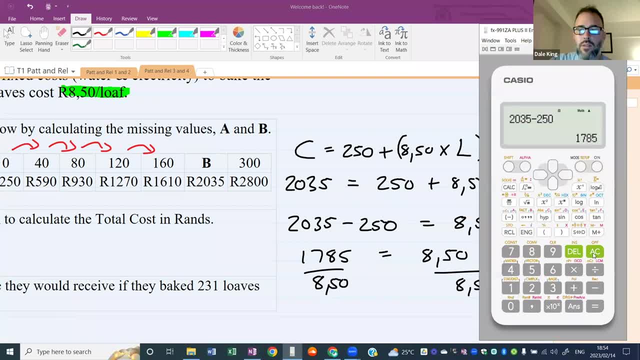 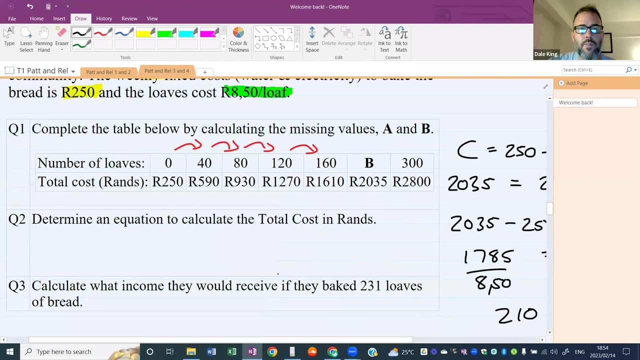 and let's see what we get. so 1785 divided by 850: 210, very good, okay. so what i'm trying to show you here is sometimes it can be dangerous to use a constant difference to find your solution. it is a possible, it is a method, especially if the question said: